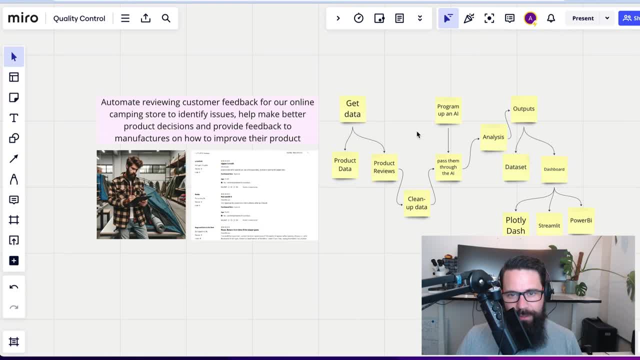 prioritize and automatically visualize and make sure that any products that we're purchasing as customers are of the highest quality And if there is an issue, we're able to quickly identify that. So, to recap, where are we at? So we were able to get some data, which is awesome. We've got some 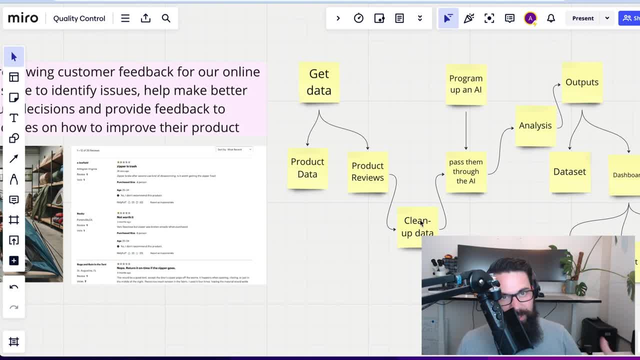 product and review data. We started cleaning that up and we're just going to finish that. right now, And in this episode, we are going to mess around with the OpenAI chat GPT API via Python, And I'll take you through exactly how to log into OpenAI, how to access the playground, how to write. We'll 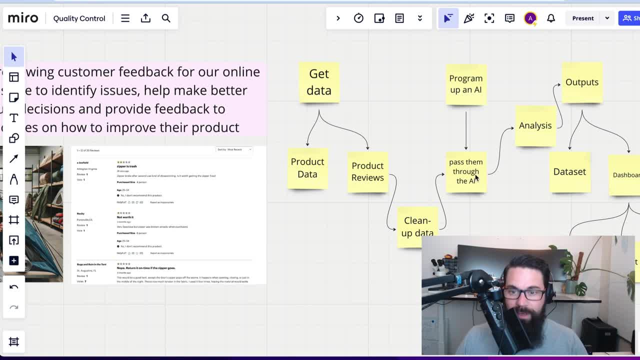 go into all that detail. after that We'll be ready for all the other bits and pieces which potentially will come in subsequent episodes. So make sure you are subscribed. We've ticked over 20,000.. So I'm just going for it: 100k, I want that. 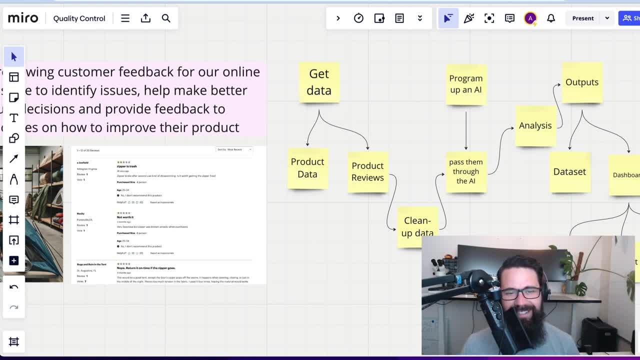 silver plaque. But if you're not subscribed, please consider subscribing. It really does help the channel. So let's get into it. First thing we are going to do is we are going to look at our very messy code, and I'll quickly recap on what that's doing, So scroll the way to the top. 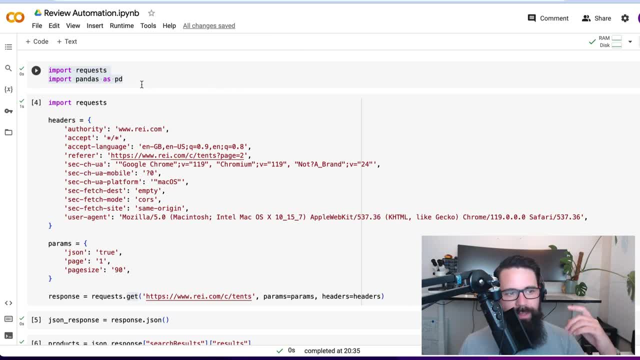 I'm in Google Colab. What we did was we were able to import requests. That helps us interact with APIs and pandas. And I imported pandas because I thought it'd be a nice way to visualize the data, especially for you watching. But at this stage, not particularly- 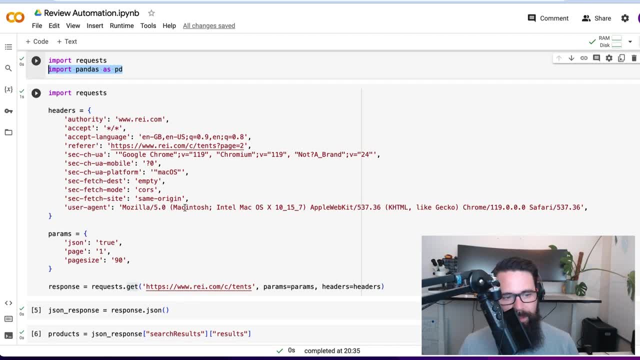 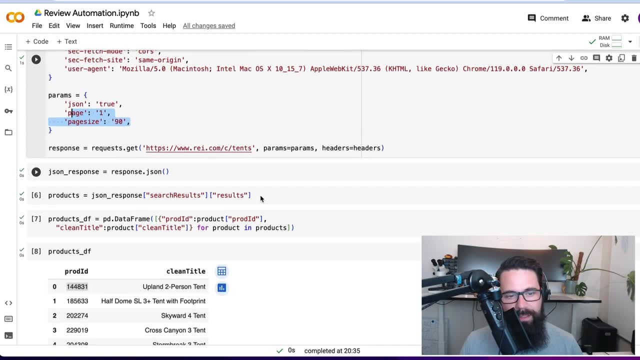 required. So the first set of instructions we've got here is a very simple API call over to the products And that's able to get 90 products. We do a small amount of cleaning through a list comprehension And then from that we get this really lovely data frame which we can interact. 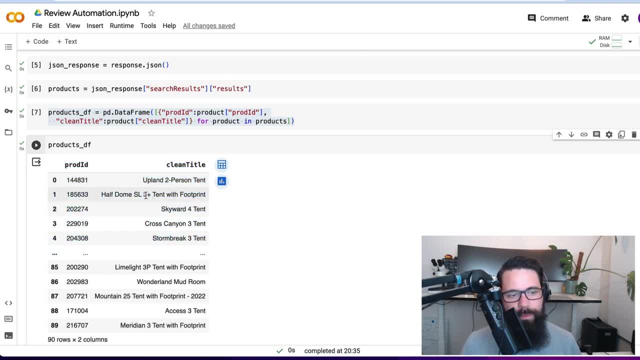 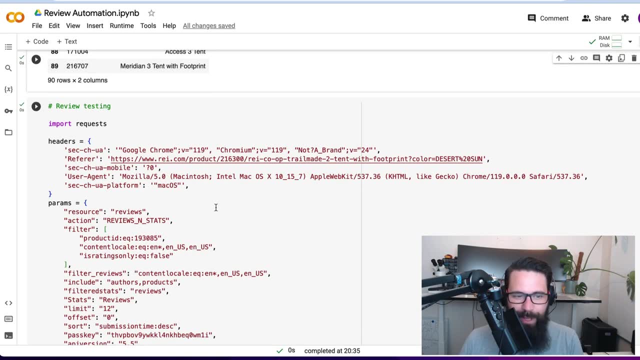 with very similar to Excel, to be honest, So keeping it really simple. And then we've got a product ID, and then we're able to pass that product ID over to this second API call, which is for the reviews, And that gives us the list of reviews And then so from that we're able to. 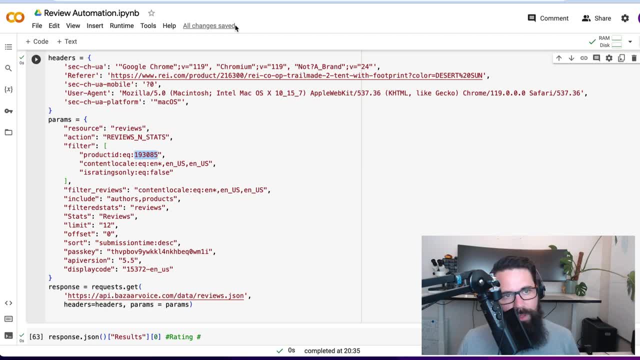 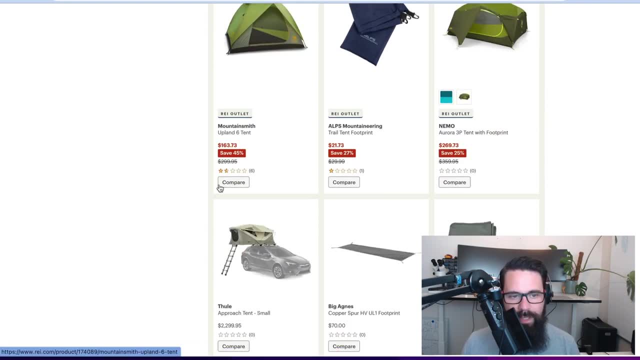 select the product ID and then get a whole heap of reviews on those products. So I'm going to scroll down and I'm going to find a product that has enough reviews for us to sort of test out with ChatGPT. So this particular product has six reviews and one and a half stars, so not the best. 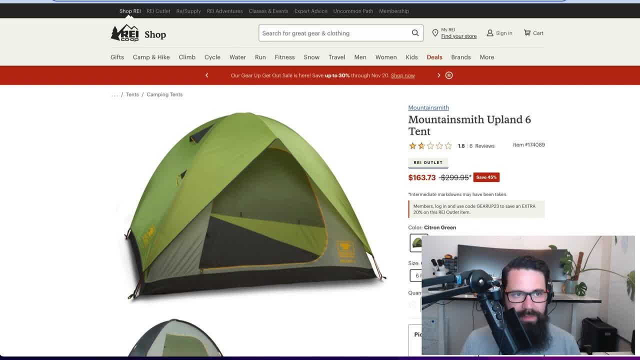 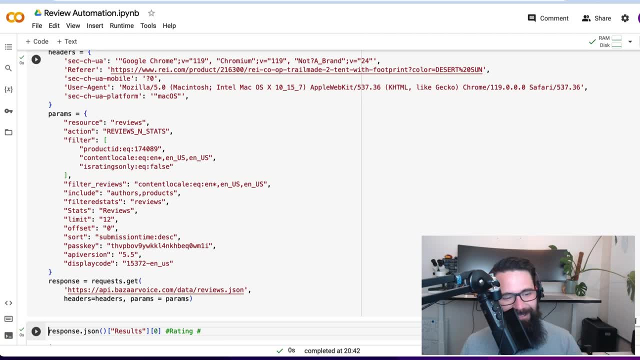 So in the URL I'm going to grab that product ID, which is there, And I'm going to pop that into the reviews API call. I'm going to shift, enter on that. That's going to run, And then from there, what? 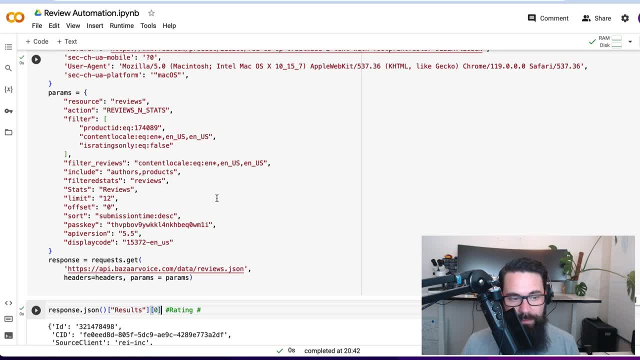 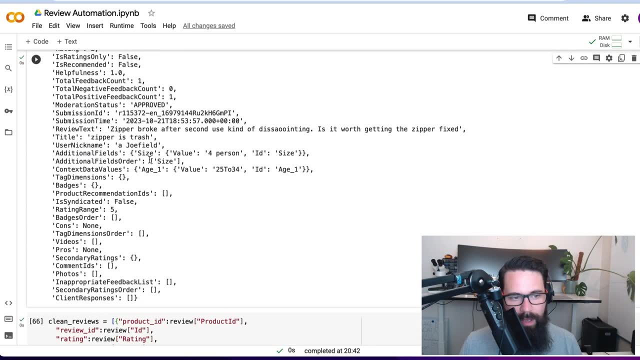 we're going to have access to is those six reviews. I'm going to look at the. well, let's actually get down to our clean reviews, where I scroll down, scroll down, scroll down. We do have to clean up this notebook, And then, from there, we're going to have a look at our clean reviews, which is this: 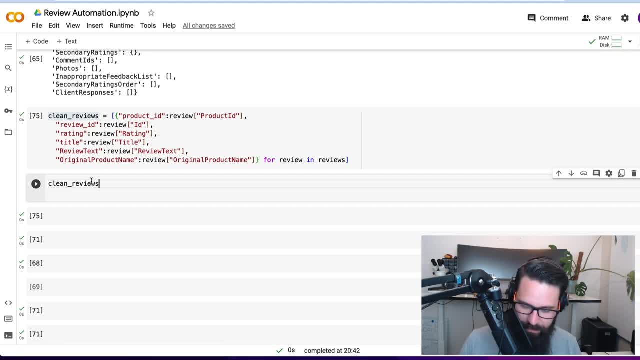 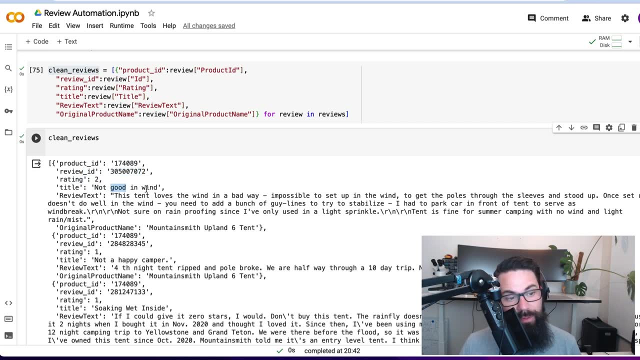 one here. So let me go ahead and click on that, And then from there we're going to have a look at our clean reviews. So let me go ahead and copy that and paste, shift, enter. Alrighty, so what we got here? we've got the product ID, the review ID, the rating, the title- not good wind- the review. 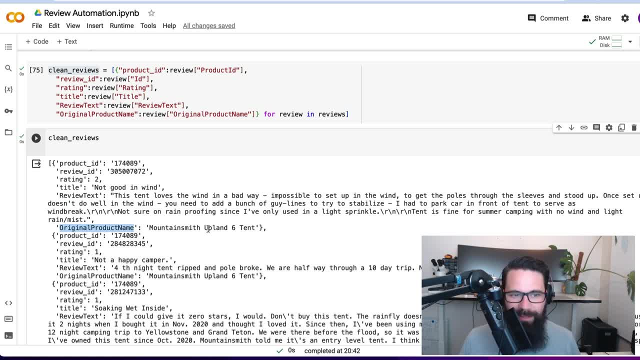 text and the original product name. So ideally, what we want to do is we want to pass part of this payload over to ChatGPT and then have ChatGPT do some categorization on all this really rich text, with some of the themes, such as: you know broken zipper, you know poor quality tent poles. 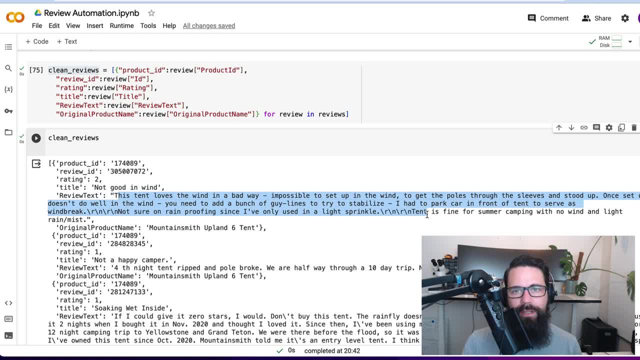 you know, whatever we can kind of get out of that information, because it becomes really useful trying to work out what's driving some of those themes and those low, one-star reviews. So how do we do that? A couple of things. I'm thinking is I'm going to get rid of product ID and review ID for 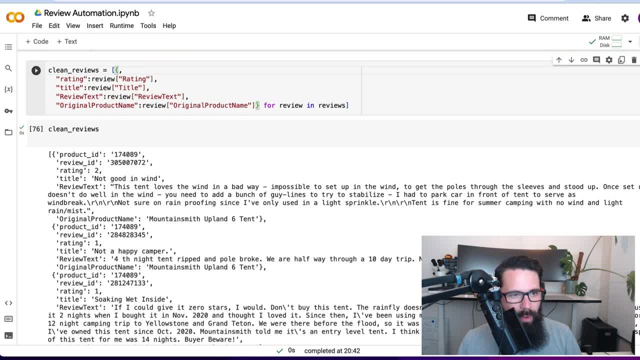 now only because we have that information, Like we've. I don't need ChatGPT to know that, like we've got that in Python. So once we pass the text over to ChatGPT, we can just add it on it. 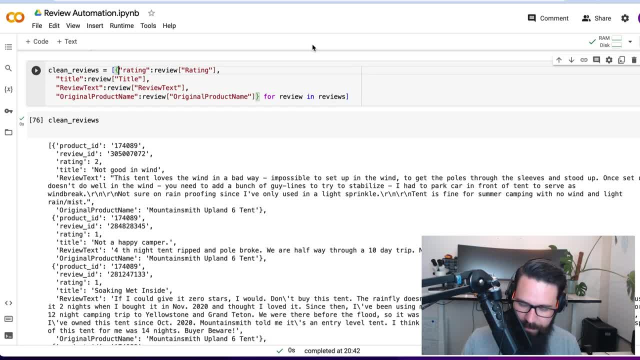 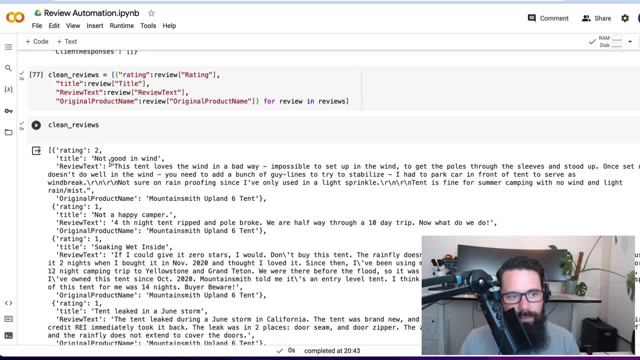 and then we can do that afterwards. So let's go ahead and leave that out for now. Let's shift enter on that and shift enter again. And now what we've got is we've got rating, which I think is quite useful, We've got the title and we've got the review and the original name. So ChatGPT knows. 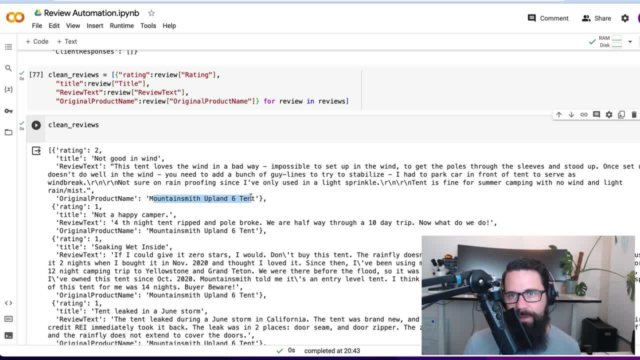 it's a tent which might be useful if we are looking at using this for other products, not just tents. So what am I thinking now? I only really want to pass over sort of low ratings to ChatGPT for testing. So let's go ahead and filter this down to the ones and twos. I have a 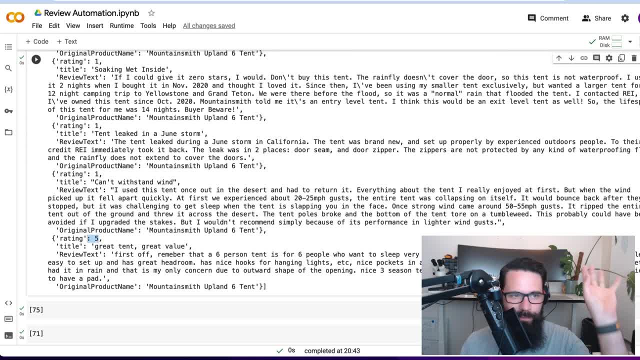 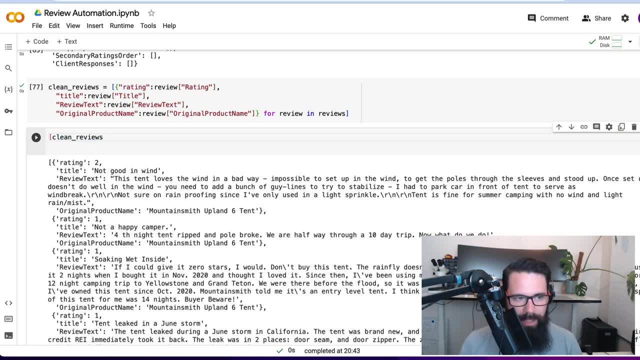 suspicion. they're all rating one. Okay, Here's a rating five. So this will prove that I'm doing this correctly To filter these out. what I'm going to do is I'm going to use a list- comprehension Now, if you recall from last time, we can say something like X for X in clean reviews and put 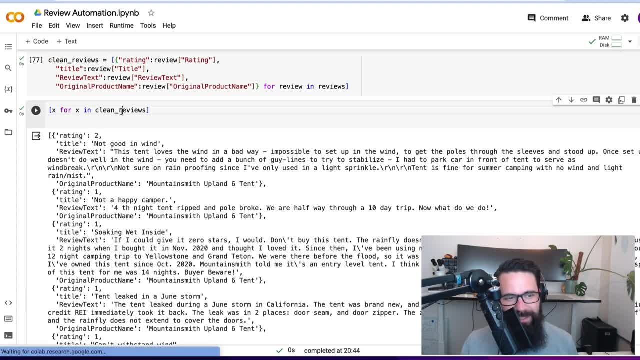 that in square brackets And when I run that, nothing actually changes. Everything's the same. It's still the same list, but now I've got access to the items in the list, What I mean by that. So X for X. all that saying I could say any letter doesn't matter, say any word, but X now represents. 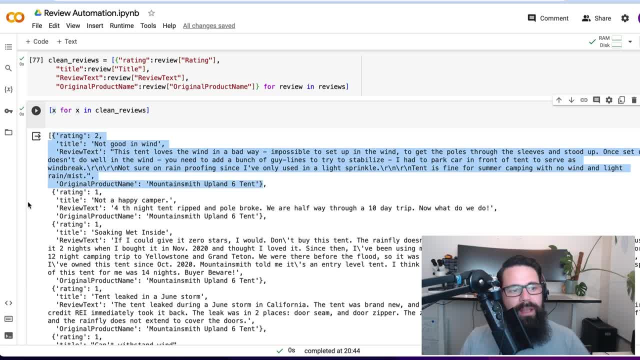 each dictionary which is between these square braces inside this list. So what that means is I now can say something like if, and we can say X, and that's now the dictionary and we can call say rating. It's not right, I've just typed some random letters. We can type rating, Okay, And 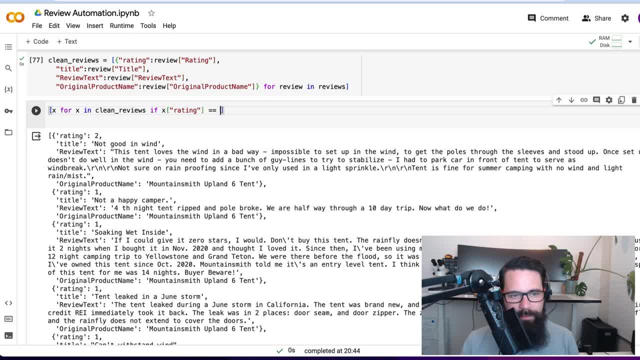 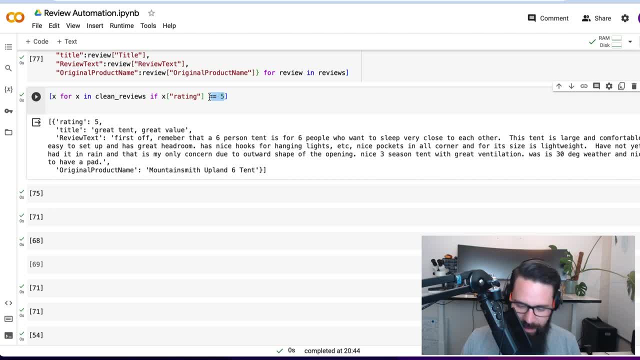 rating. let's actually test this. Say rating is equal to five and we should only get the rating five back. Perfect, And then what we'll really interested in is all those that are less than three. So we've got ones and twos, which now gives 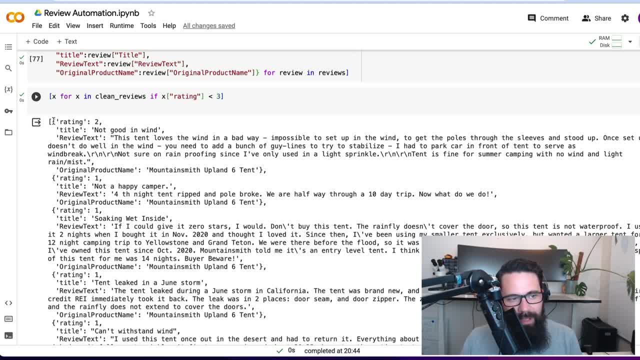 us these ones here. So what we want to do is we want to basically have these Python dictionaries in a string or JSON object format, which we can do in Python, and pass that over the chat GPT, have it interpret that text and come back to us with theme. So to do that, what we'll need to do, 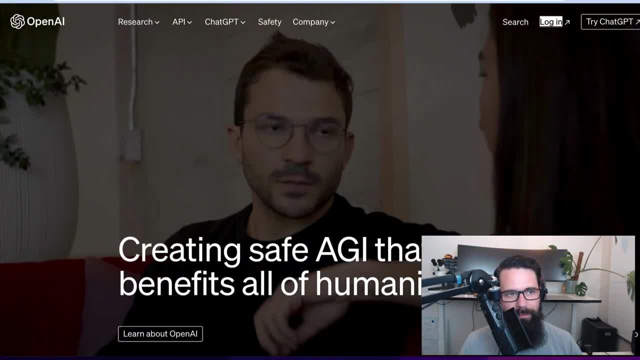 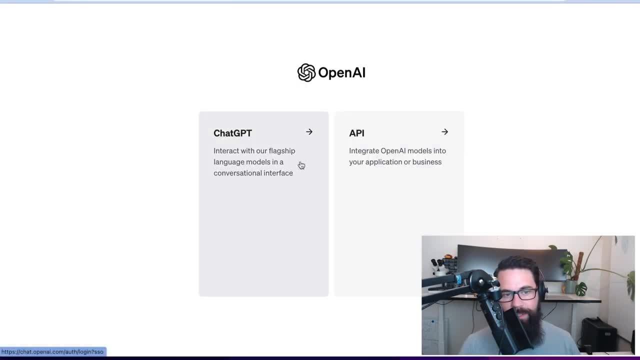 is, we will need to log into OpenAI. So head over to openaicom and then, on the right-hand side at the top, hit login. From there you got two options. You might be familiar with chat GPT, which is fairly popular these days, but we're 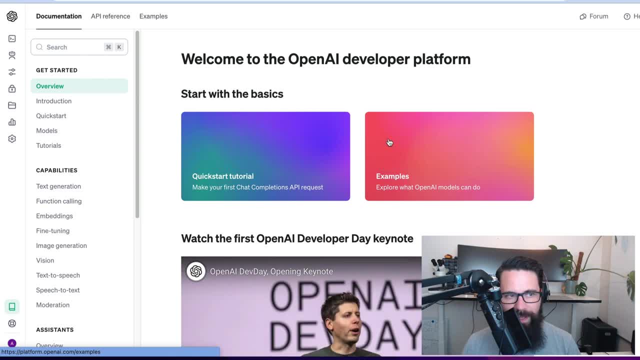 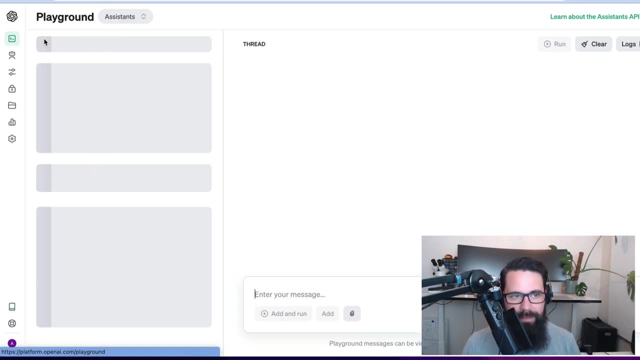 actually going to go to API From there. on the left-hand side, you've got playground or assistance. We are going to use playground today, but I'm looking forward to playing with assistance as well. So I'm going to hit playground And then from there, what we've got is: where is it? Okay? 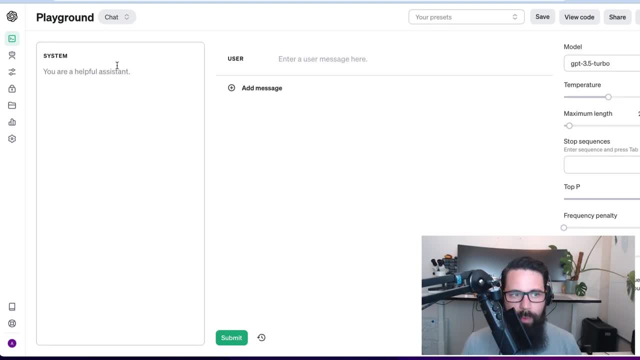 cool. So here we are In the playground And what we've got is: we've got our system message, And our system message is really what we're kind of instructing chat GPT to do. So, for example, we could say: you are a. 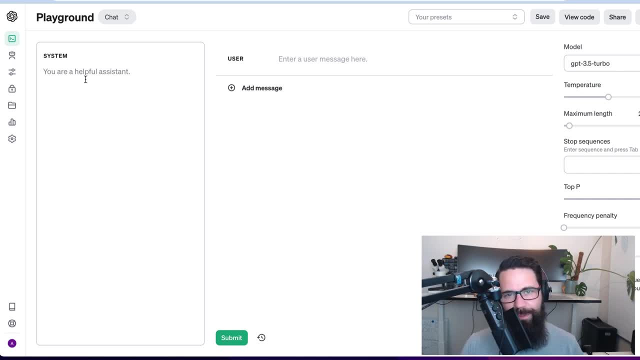 helpful. you know, product review categorizer, You'll return a list of themes in a valid JSON format, because then we can interact with it in Python As a user. we can then give it the JSON payload, which is our review sort of text and a review description, And our expectation is: 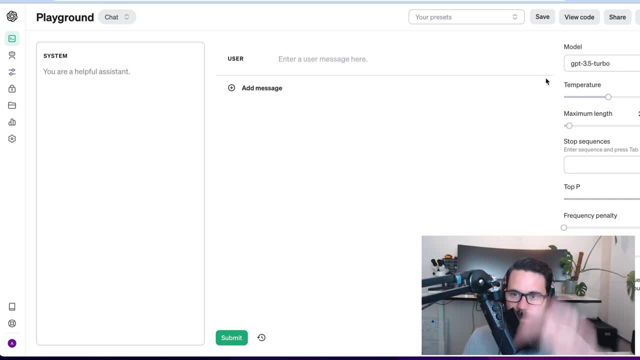 that it will return that valid JSON object. Now the options on the right-hand side are around the model that we'll be using. I'm not anticipating a huge amount of text. I'm going to leave everything fairly standard. but have a bit of a play because, depending on your system message and your user, 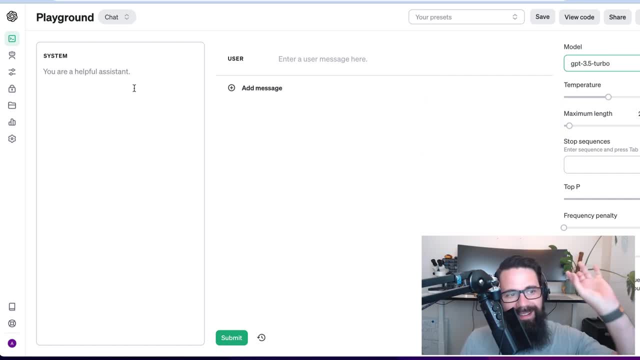 messages, these sliders will behave differently, So let's start with our system message. Now we want to say something like. you will be provided a product review In the following JSON format, and we'll pop our format in there once we get hold of it. 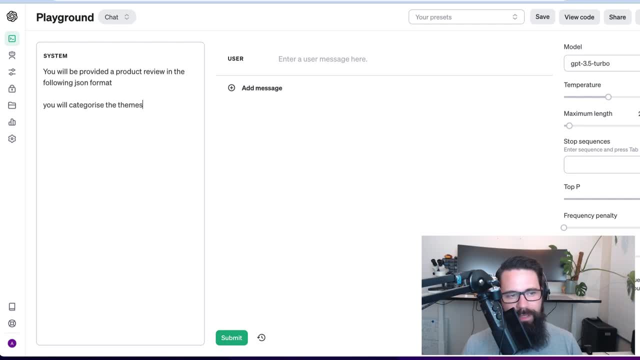 You will categorize the themes. you'll be provided a product review in the following JSON format: You will categorize: you will categorize the themes related to the review outputted in a valid json format. like so, perfect. so first of all, we need to give it a json payload now. unfortunately, 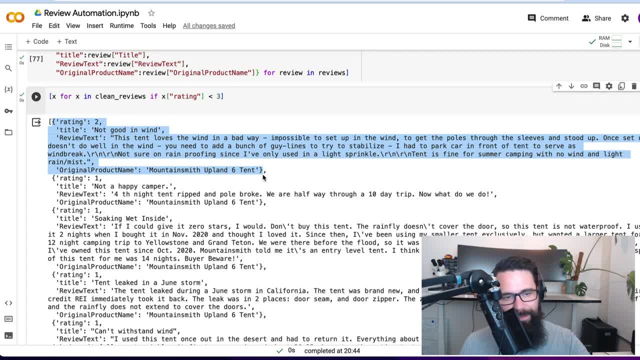 we have those on hand now. if i was to copy and paste this particular payload, uh, it isn't actually valid json. it's very close, but it's actually a python dictionary. the main problem is it's using single quotes and not double, but the good news is python has a package for that, so we can import. 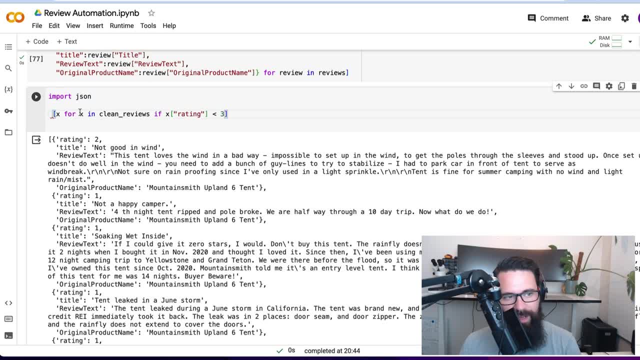 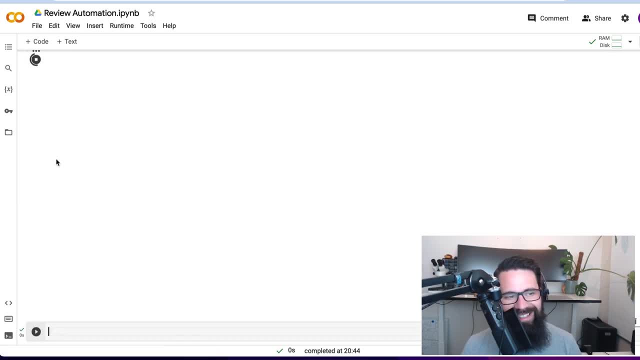 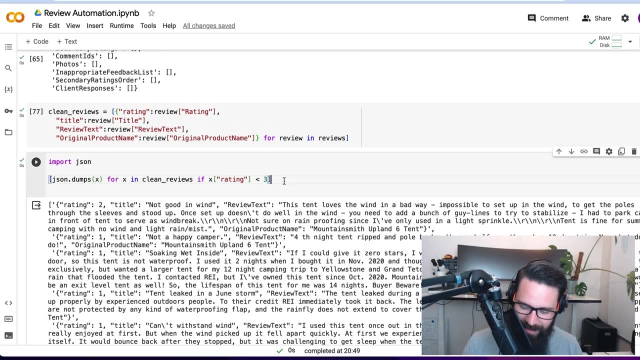 json, and then we can say inside our list, comprehension. we can say json dot dumps, which is a bit of a funny one- shift, enter on that, and all that's done is, rather than having python dictionaries in our list, we've now just got strings. so what i mean by that is if i was to say: 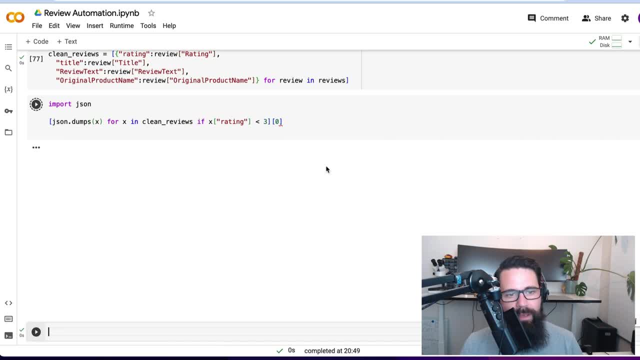 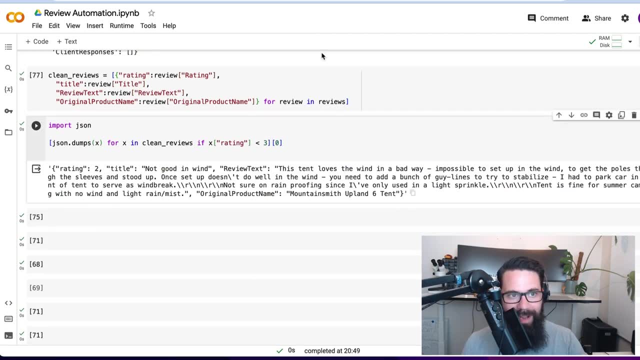 give me the first item in our dictionary shift: enter on that. you can see here. it's in single quotes and if i was to ask for its type it would actually be a string. so i'm going to copy that out. i haven't read too much about it because i want to see kind of what it comes back with. oh, actually, no, sorry, i take that. 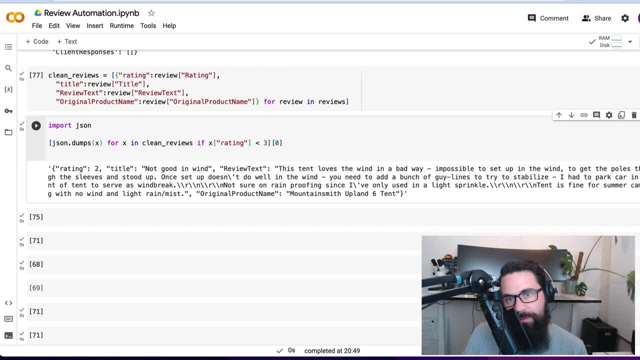 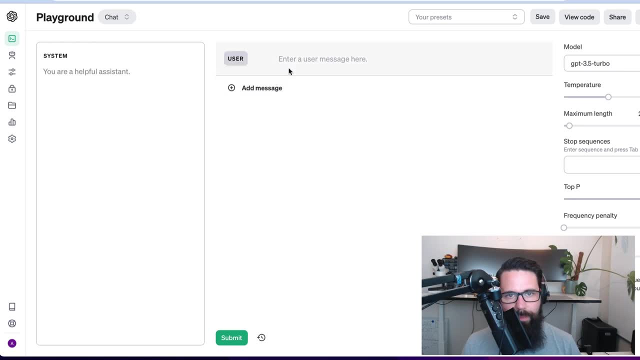 back. we need to read this one and give it a bit of a hint on what the things we're looking for, and then we'll give it the next review to see what it comes back with. so to do that, let's go ahead and paste: oh, where am i? oh, here, it is okay. you'll be provided a product review in the following json. 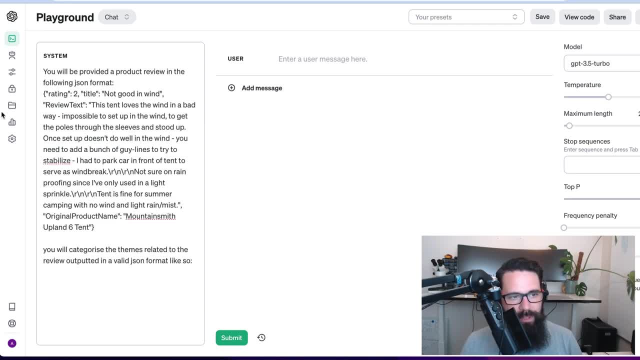 format, so let's paste that in here, which is oops rating. to title: not good in wind. uh, this tent loves the wind in a bad way in possible to set up in the wind, to get the poles through sleeves and stood up. i'm not gonna give. 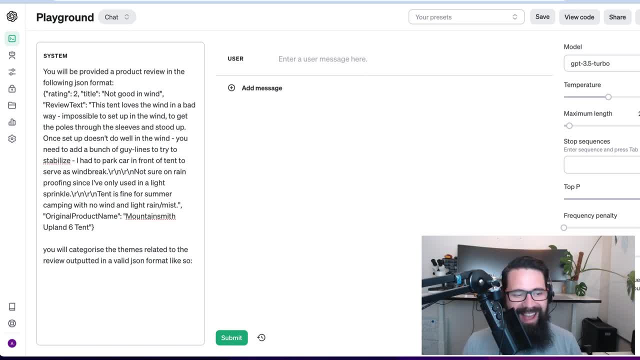 it too much back. in fact, i'm just gonna ask for it to give me back- um, let's have a look. so ask for it to give us back maybe a json payload that has a like a key called themes and then maybe just like a list or, as they're called, arrays of different themes, so we can just say theme one and we'll. give it theme two, and i'm not sure if that's the right way to do it, but i'm going to give it theme two. and i'm not sure if that's the right way to do it, but i'm going to give it theme two and i'm not. 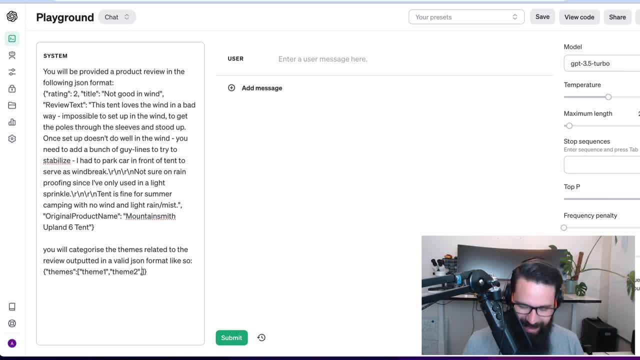 sure if that's the right way to do it, but i'm going to give it theme two and i'm going to give it that's going to encourage it to just give us two themes we're about to find out, and then we'll give it theme oops, theme three. okay, now that's awesome. so what have we done? 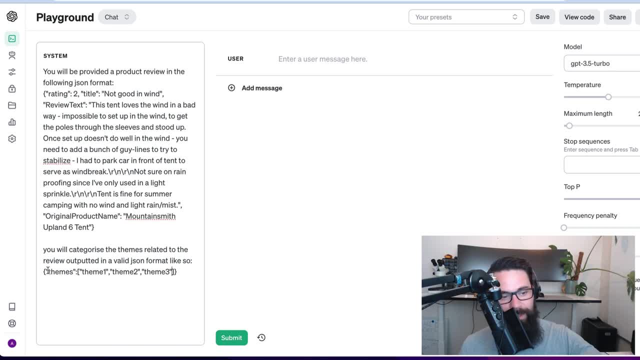 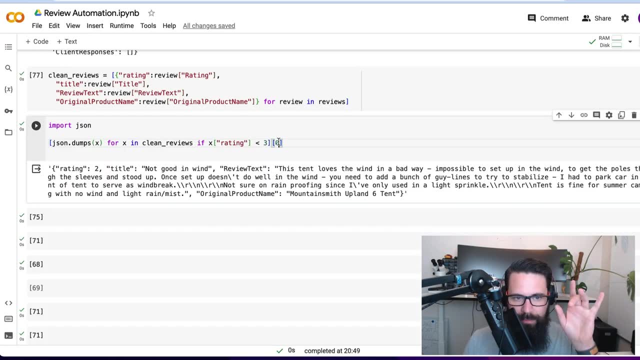 here. so we've basically said: this is what you're getting, this is what we want returned. now let's test it. so to test it, all i need to do is pop back into my python and rather than go to item one or list- you know, item zero, which is the first item in my list- i'm going to go to item one, which. 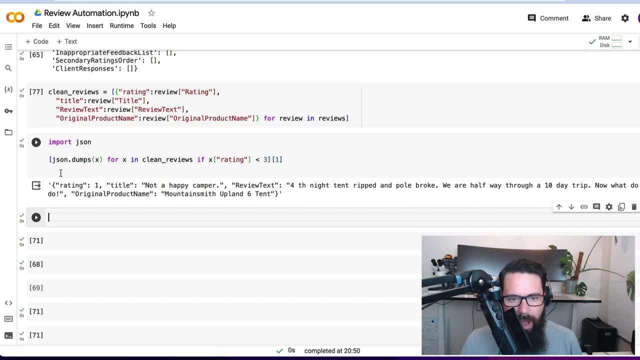 is the second. and now i've got a new json payload and i'm going to go to item one and i'm going to load. i'm not going to look too closely at what it's saying. i'm going to hopefully see what chat gpt comes back with and then we can go through and kind of review it's working out. so let's go. 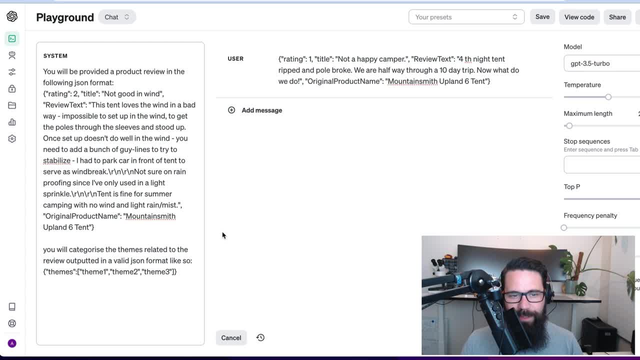 ahead and paste that in there and let's submit that and hopefully first of all we're looking- it will come back with a valid- uh yeah, valid- json object, which it has, which is great. it's, like you know, curly braces, square um brackets, and it's saying durability and quality control. let's have 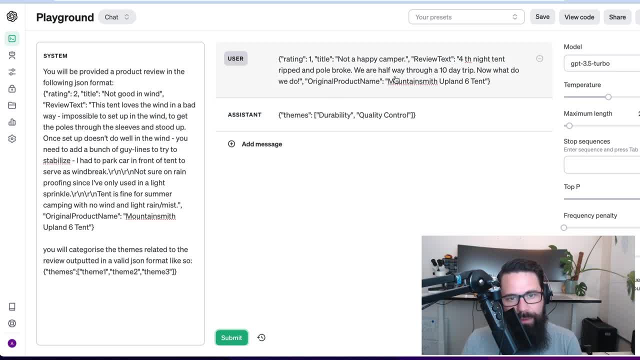 a look, not a happy camper review text. fourth night intent ripped poll broke. um, we're halfway through a 10-day trip. now what to do? okay? so is it durability? is it quality control? yes, they're pretty broad topics and we can probably get a bit more detail. 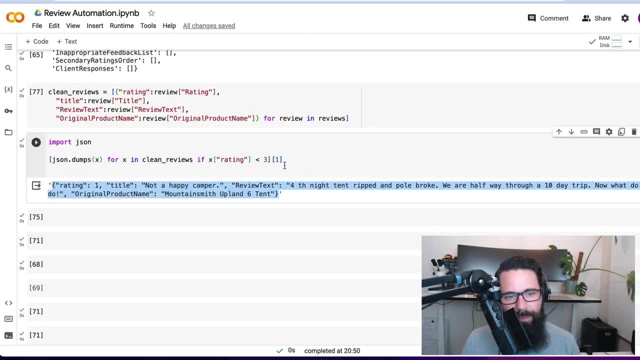 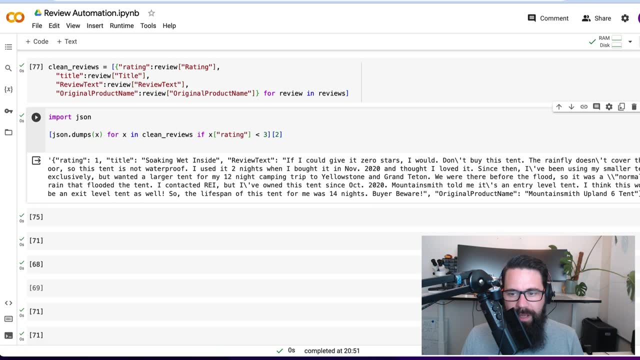 but let's not do that just yet. let's try another one and let's see if we're happy with this sort of broad sort of topic. so let's go ahead and go for the next one, and we are going to copy that out and let's paste it in. where are we pasting in here? okay, and let's go on that one. 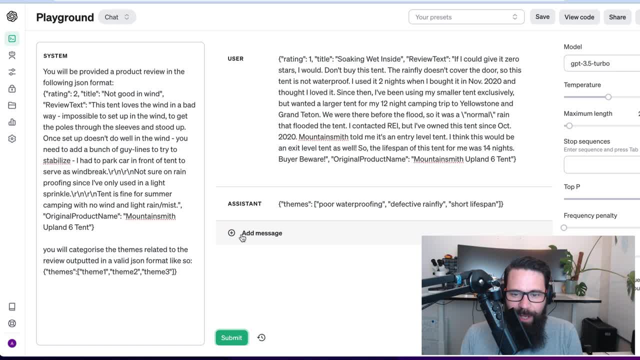 okay, waterproofing: defective rainfly, short lifespan. there you go that's. that's pretty cool. that's pretty cool, okay, all right, i'm kind of happy with that. so we've got our system message. we've given it a user message. it's come back um with its response. so to make our lives even easier, 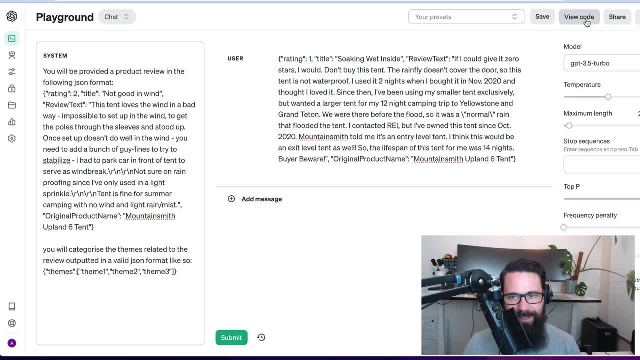 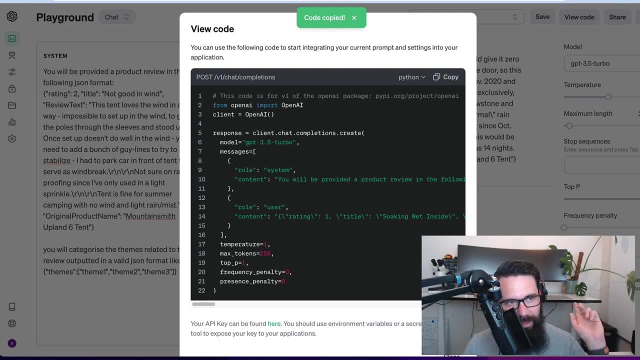 let me get rid of that one. what openai has available to us is the view code, and it's going to give us some python code, all right. so what i'm going to do is i'm going to copy out that python code and we're going to talk through it, so it's not all going to be just copy and paste. 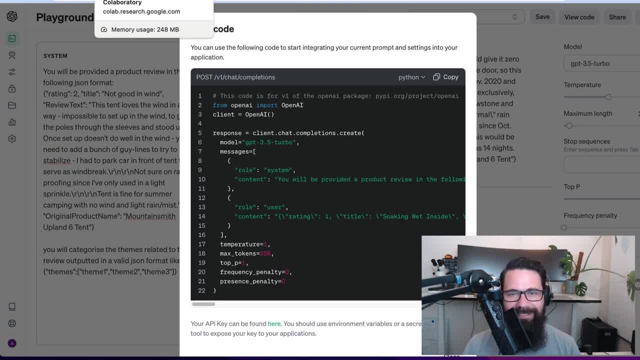 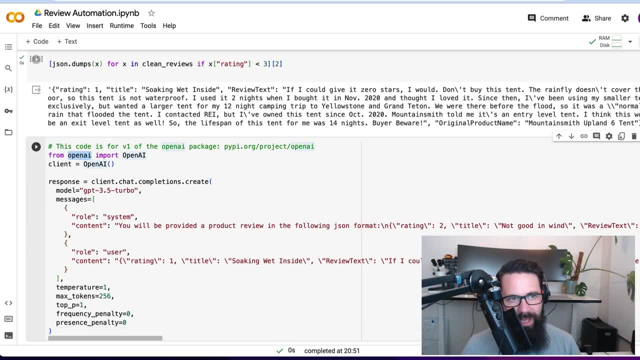 code, because i'm not a fan of that. i've seen reviews. people like here's some code and you're like what's it doing? so, uh, let's paste that in first thing we are going to need to do is we are going to need to install openai to do that, to double check, head over to pypiorg, uh, and double. 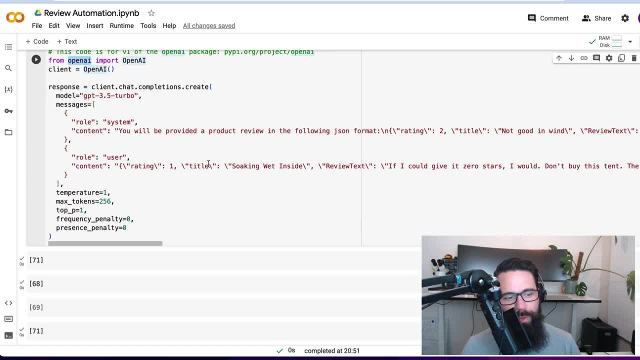 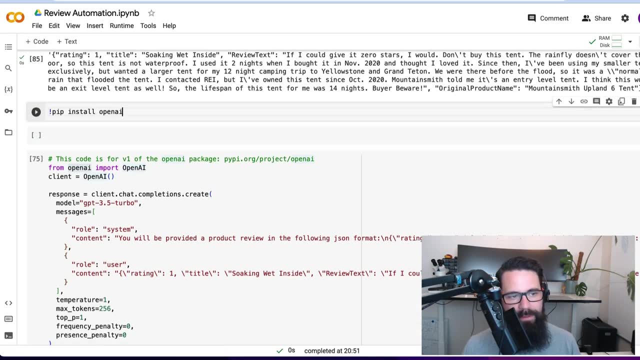 check that we're installing the right package, so let's copy that. now we are in a notebook, so we can actually go ahead and let's give ourselves a bit more space here. we can actually say that we've installed openai and we're going to go ahead and install it, so we're going to go ahead. 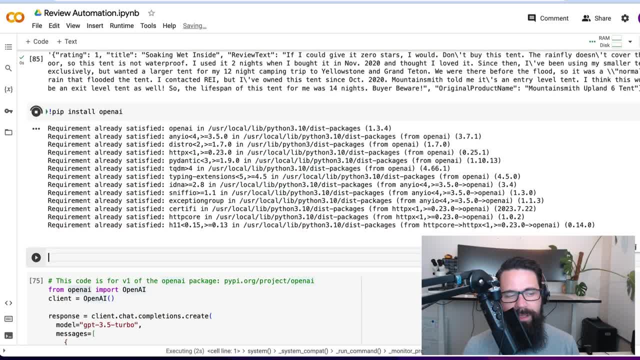 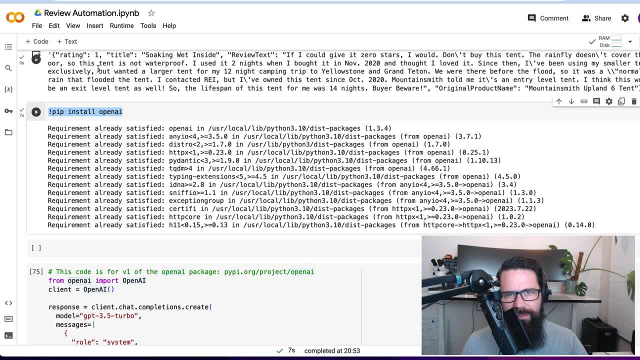 and install it. so we're going to go ahead and install it. so we're going to go ahead and install openai. now, i think this one might already be installed. yep, that's already been satisfied, but if it wasn't, it will go ahead and install that for us. if you do the install and it doesn't run. 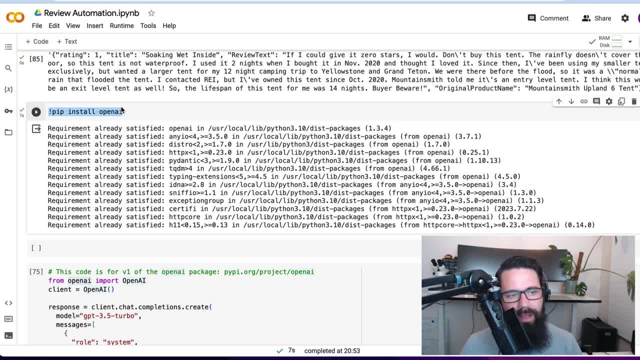 straight after, like when you say you know from openai, import openai. you may need to head up to runtime and then restart. your kernel might not have detected it, so shift, enter on that, let's scroll down and let's get a feel for what we're working with here. so 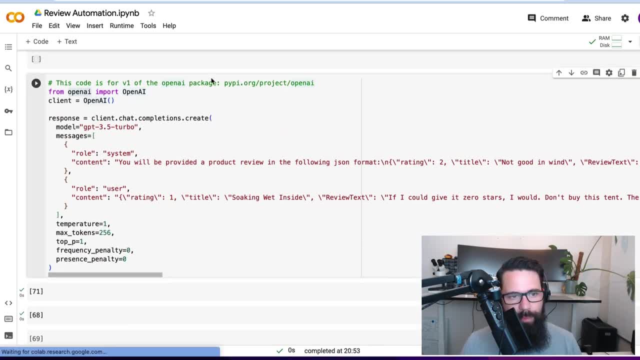 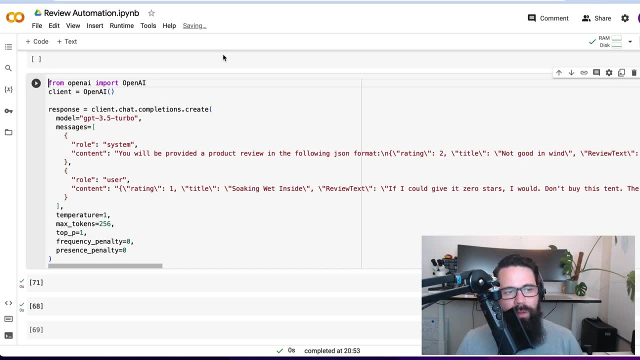 first of all, it's saying the code is v1. boom, boom, yep, check your openai. okay, cool. so from openai, import openai and we've got a client here now we are going to have to pass in api key now, as we can do a whole video on how to handle secrets and api keys and the best advice. well, actually i'm going. 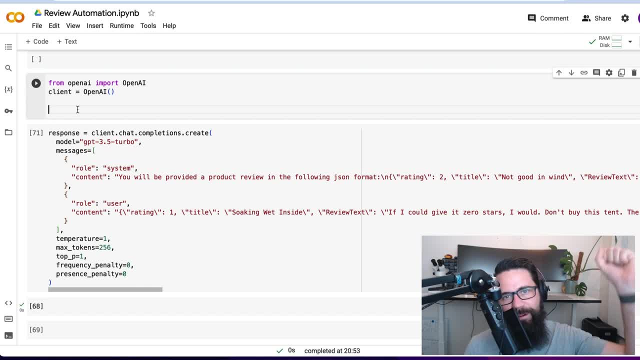 to be honest with you, everyone's got a different point of view on this. some say environment. i don't know. don't even know how some people do it, but working with api keys is always a bit of a risk. so what i'm going to do to make my life a bit easier, i'm going to show you how to get your api. 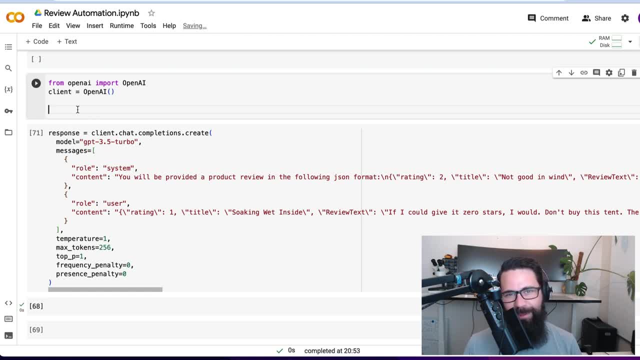 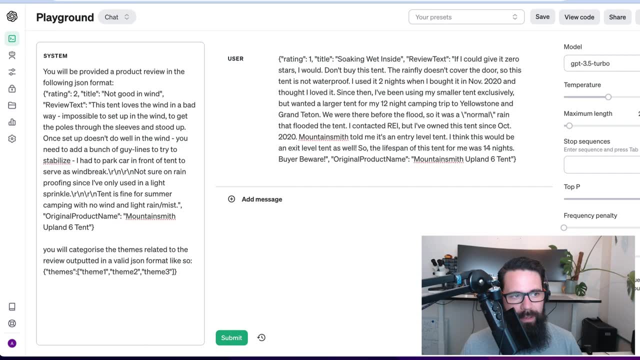 key. that will be shown on screen and then, shortly after recording this, i will delete that api key. and, if i forget, you got yourself a free api key, so let's do that now. so let's head back to our playground. over on the left hand side we've got api keys. we'll open that up over here and here's. 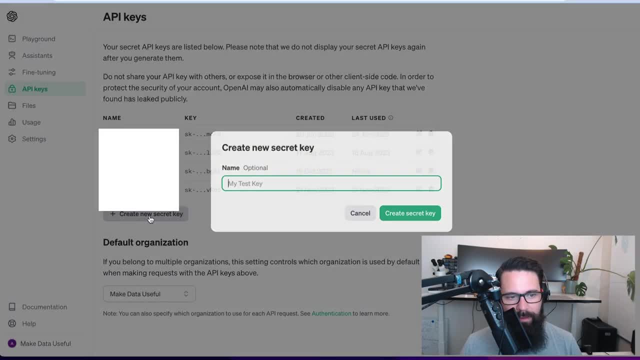 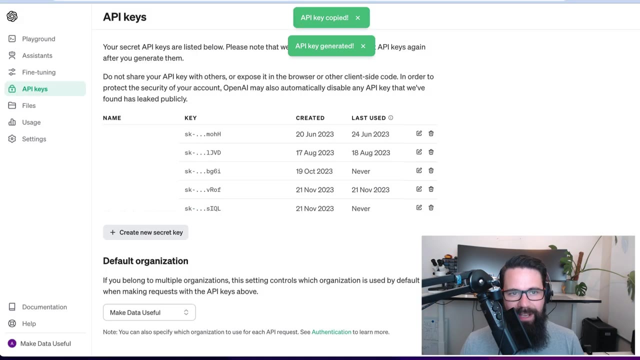 a list of my api keys for a whole bunch of different stuff. i'm going to go create a new secret. uh, i'm going to call this one tent review. where are you? tent review automation. okay, i'm going to create that secret and i'm going to copy it. now what i can do is i can add that as an 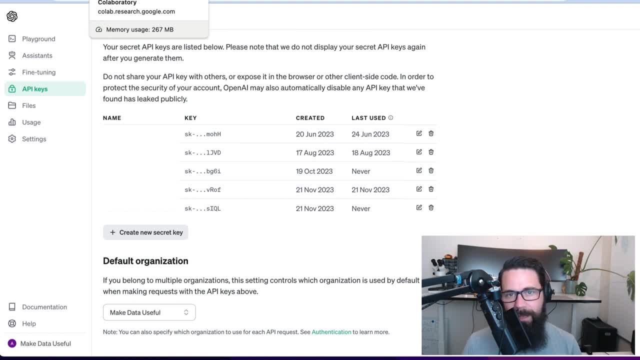 environment variable to my system through the terminal. if i'm in windows, um, you can obviously google this or use chat gpt, but you can use set x and on mac there's a few different ways. you can do it through your shell, but for simplicity and because i'm using google colab, 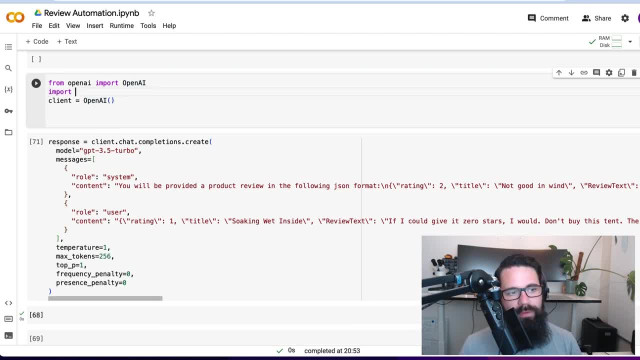 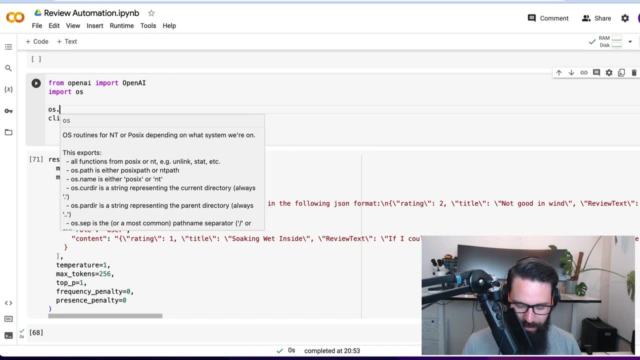 what i might do is i might import the os package and again, this is not the recommended way to do it, so make sure you search the best way for you to do this. but i'm going to say osenviron, which is basically the ability to set an environment variable. okay, that environment variable is going. 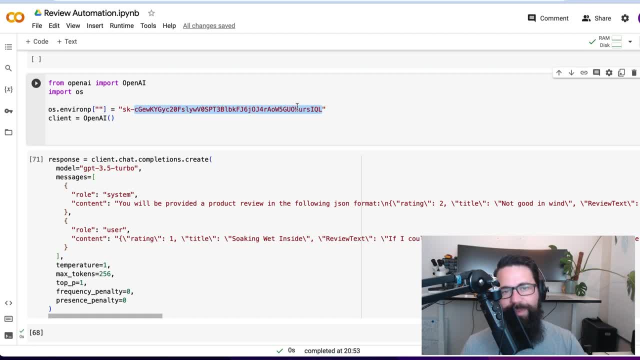 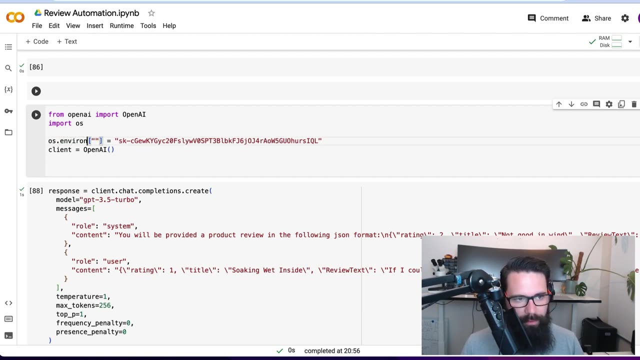 to be equal to my api key and hopefully i've remembered to delete that. otherwise you can quite literally start using my keys, which is what they want to avoid. we need to set that to an environment. that's not even right. so environment environ- perfect. now i need to set that to. 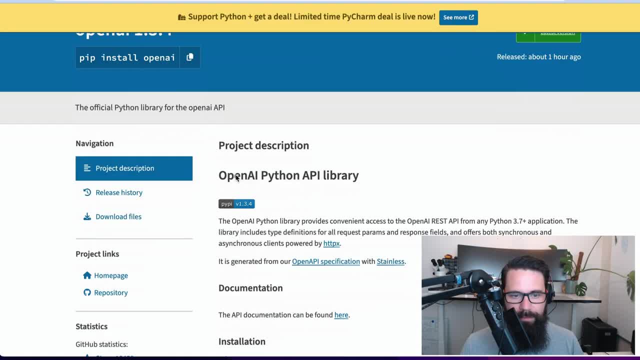 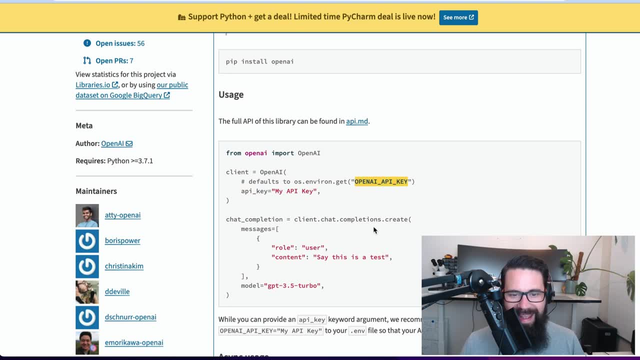 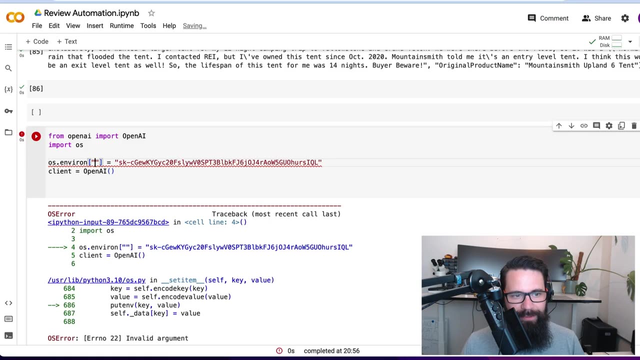 something. now that's an invalid argument, nothing. so if i head over to the documentation for the open ai api keys, a couple different ways you can set it: uh: open ap, open ai underscore, api underscore key. um, perfect, so let's go ahead and set that which is this one here and we are now shift. good, 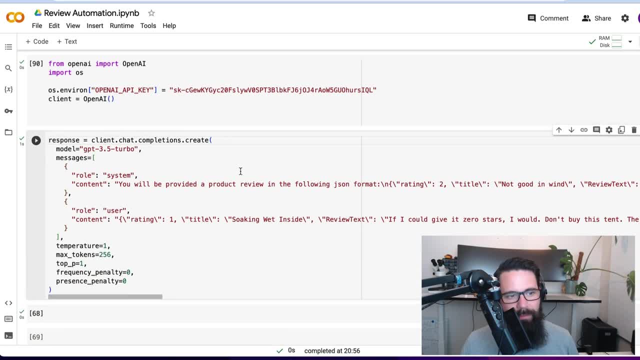 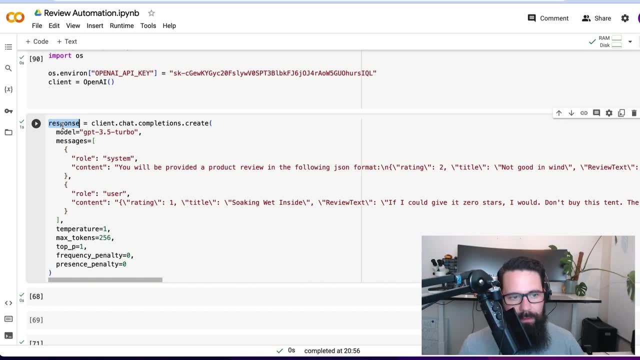 to go. so what is this code actually doing? so if we have a look at it first of all, um open is created a variable called response, which is pretty common for any sort of api call. in this case called response, it's calling client chat completions create. so it's creating a completion and just. 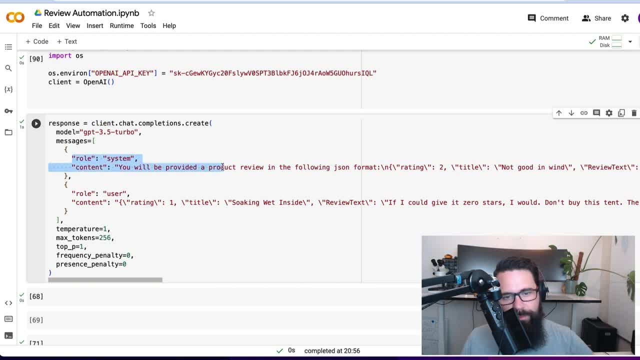 like we saw in the playground. it's no different. we now have our role, which we've already set up, and we can modify it here if we wanted to, and we've now got our user, which is our json payload. so what we can probably do is to make our lives. 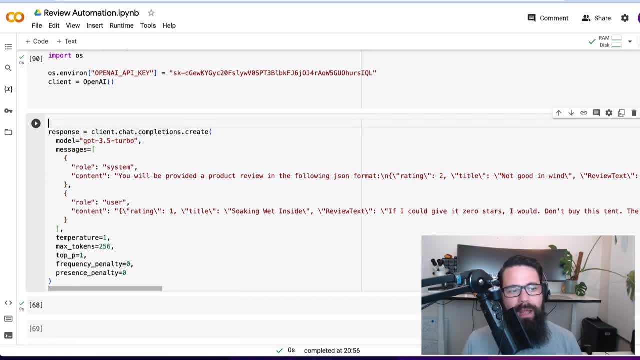 even easier. what i might do is i might wrap this up in a function, um, and we can have our json payload be passed into that function. so our review goes into the function uh. and then this responds: uh, with what chat gpt tells us. so to do that, what we'll say is: we'll say define and we'll say what. 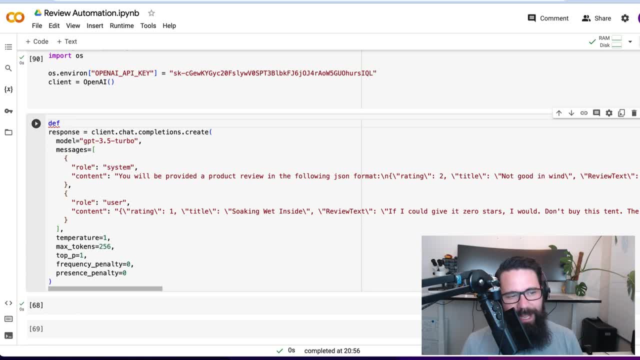 we're going to call this, uh, categorize review. it's a bit of a funny name, isn't it? so let's go review underscore themes. okay, uh, define review themes and we're going to pass here in- we'll call it, review json string. okay, just to make it extra clear. that's what we're talking. 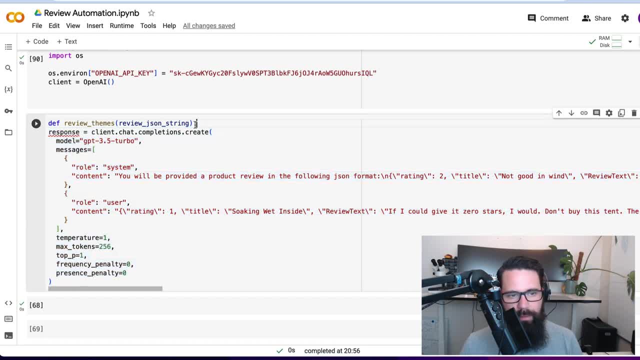 about and we're going to go ahead. put a um, what do we call? it's going to call a semicolon, it's colon atom. put a call in there and we are going to return. do i want to return everything that's returned from chat gpt? look, to be honest. for now it might just be a bit easier, so let's go ahead. 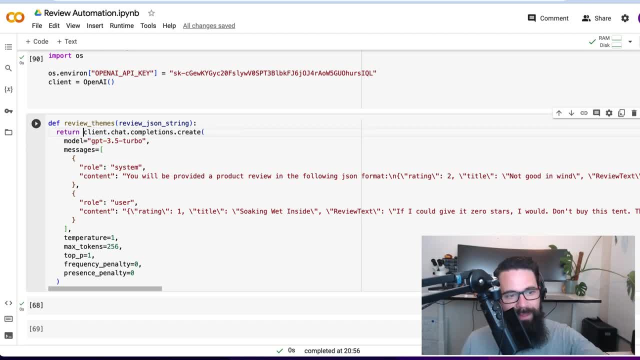 and do that. so let's go ahead and type return, and when i run this, it's going to return whatever chat. what you might have noticed is we need to replace our user content. so, again, this is really just what we're looking at here: got our system, we've got our user and it, and the same thing's happening. 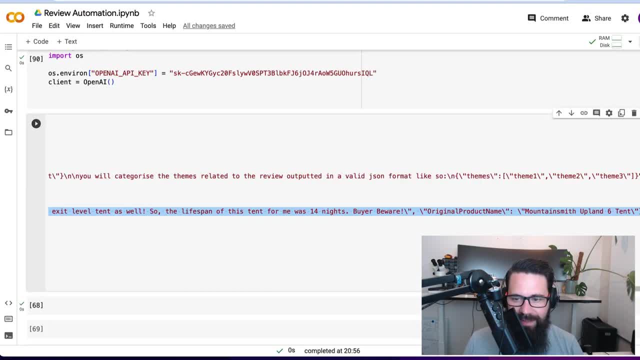 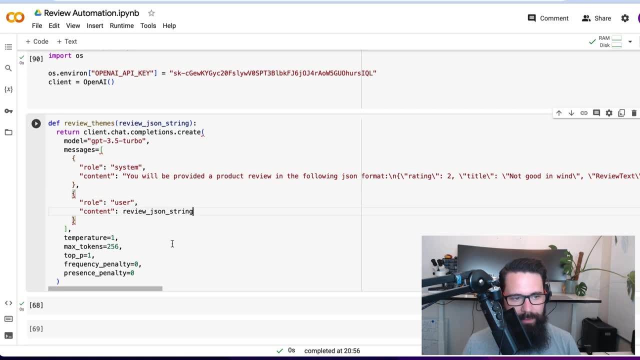 here. we've got our system and we've got our user, so let's go ahead and get rid of this text, because we don't need that text anymore, because our text is going to come from review json string, which is that one there, and we'll be able to shift enter on that. now, if i have review theme, 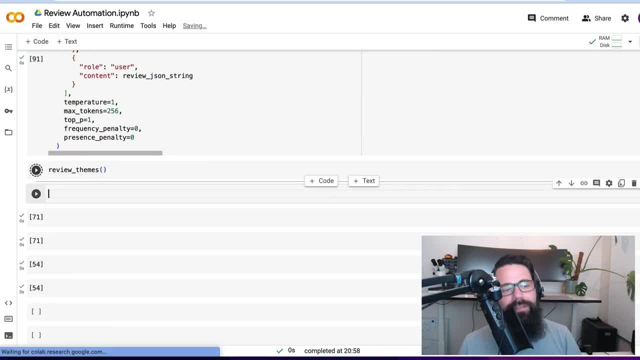 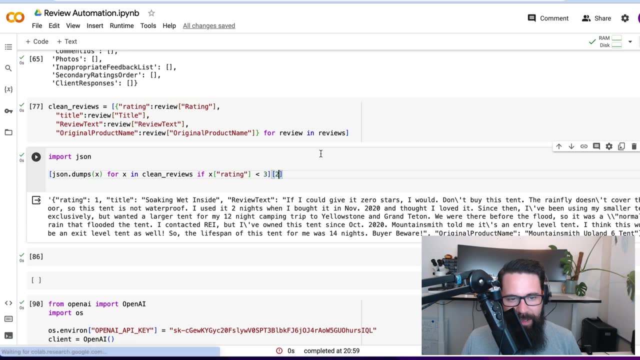 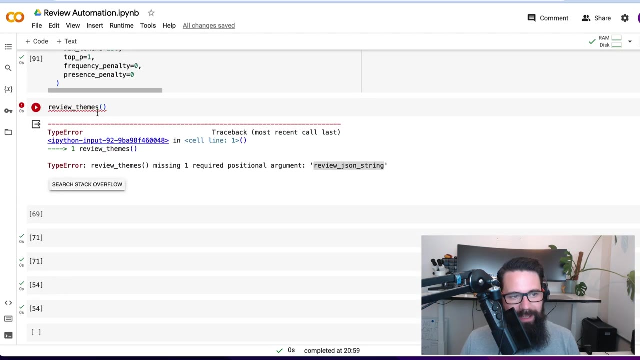 okay, and i try to run that. i should get an error saying you need to pass in. you need to pass in your review json string uh, which will be one of these, so why don't we grab another review? okay, so maybe number three here. okay, let's copy that, uh, and let's just not paste it straight in here. 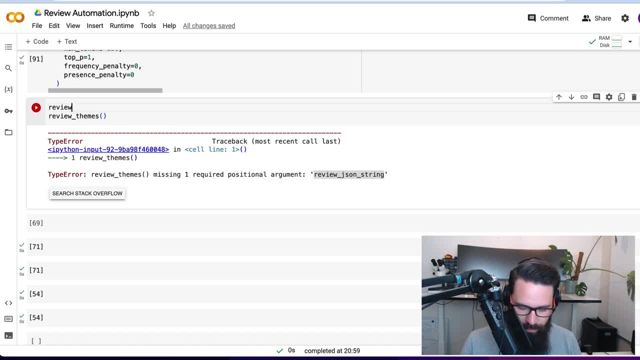 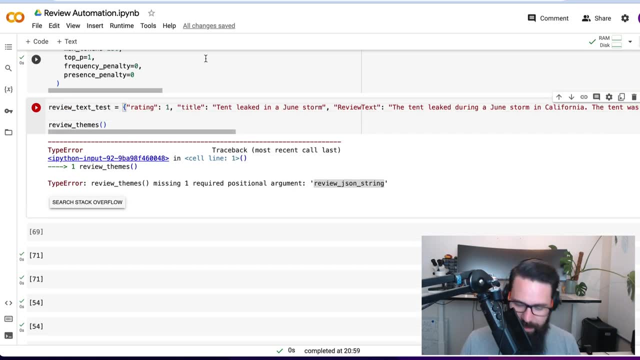 because that's a bit messy. so why don't we say: review text test: okay is equal to this particular json string string. so we'll put that in single quotes to make sure it's still represented as a string, because that's what the open ai is asking for, and then i can just pass that into here. now we can assign. 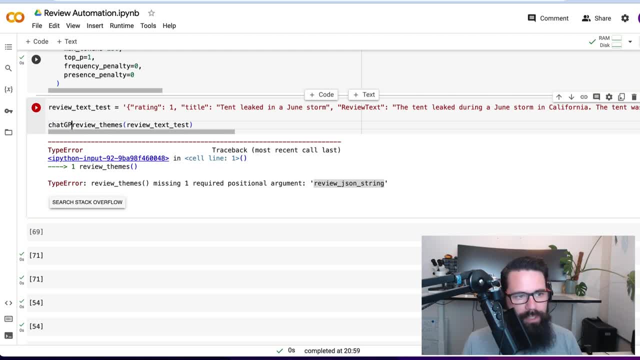 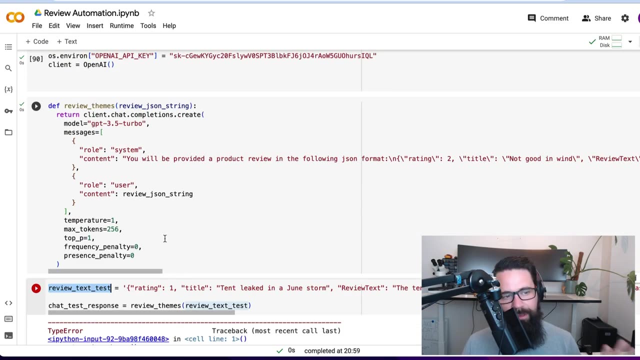 that to a variable so we can say chat gpt. oops, yeah, we'll say chat underscore. test response is equal to review themes and we're passing in our review text test. okay, it's a bit going on here, but just to quickly recap, we've created a little bit of a string here and we're going to call it a. 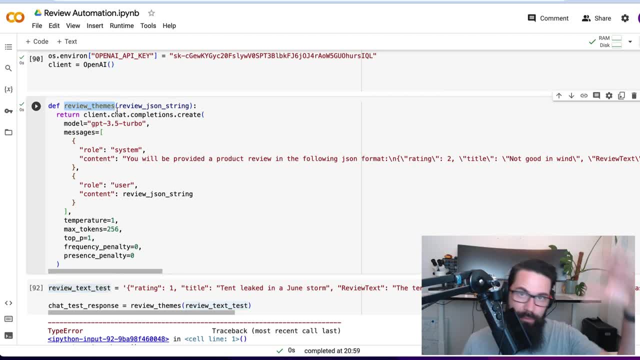 function because we want this to be a reusable code, which we're going to do all throughout our analysis. a function gets to return something and we are returning everything that chat gpt will give back to us. but when we are asking chat gpt this question that you know you'll provide a product, 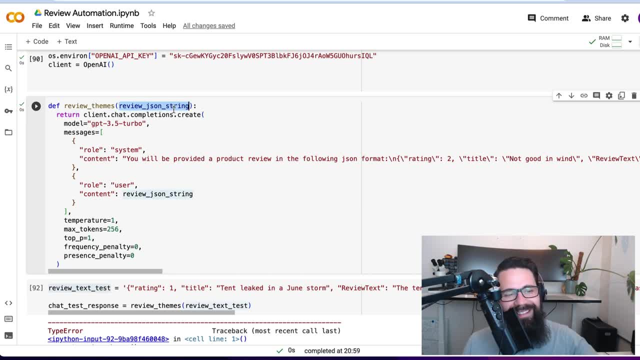 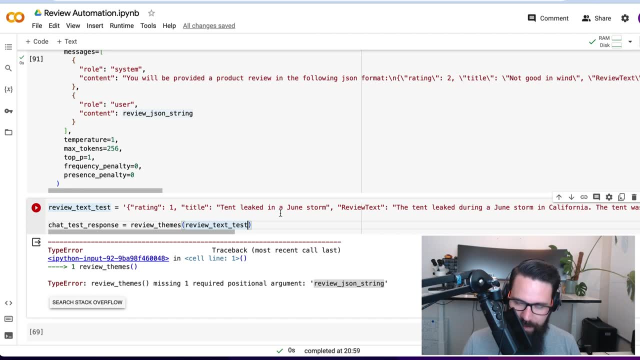 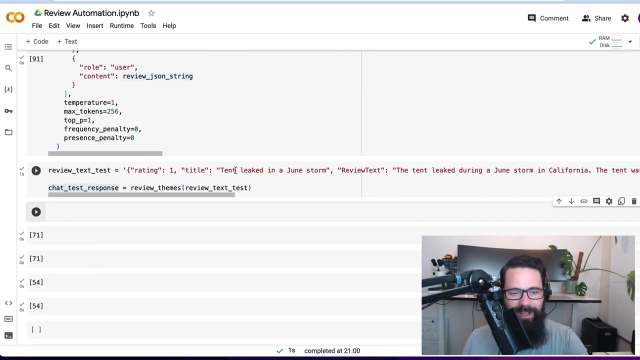 review. we've given an example. um, what if we pass in is our review json string? it will return the chat completion or the themes it's come back with for that. so if i shift enter on that off it goes. we've got a response. i'm a little bit excited. i haven't even read the full review. it sounds like. 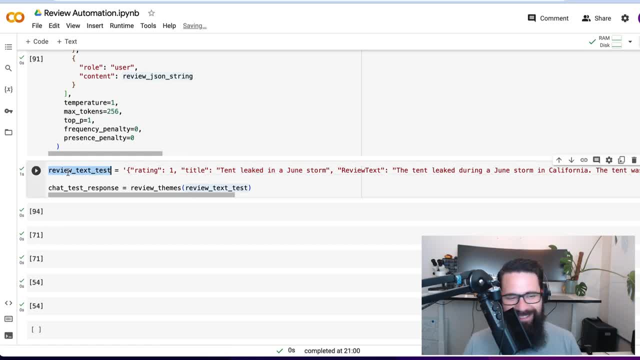 it's leaky, but you know, let's find out. enter on: oh, i didn't, didn't put anything in there, so, chat, i'm just, i'm too excited. uh, now my copy. i need to get a new keyboard. any recommendations on keyboards? put it in the comments, because i'm yeah, and this one isn't working for me. uh, shift enter. 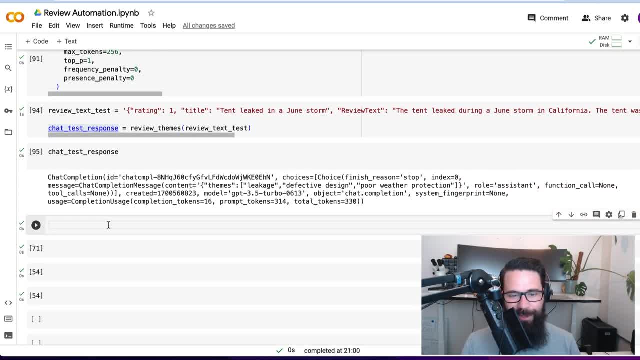 on that and what do we get back? okay, so, first of all, we've been returned a chat gpt object. okay, so this chat gpt's object, we need to sort of interrogate this. i can already see that we've got the contents, but we need to get to that content. so to get there, what i need to do is i: 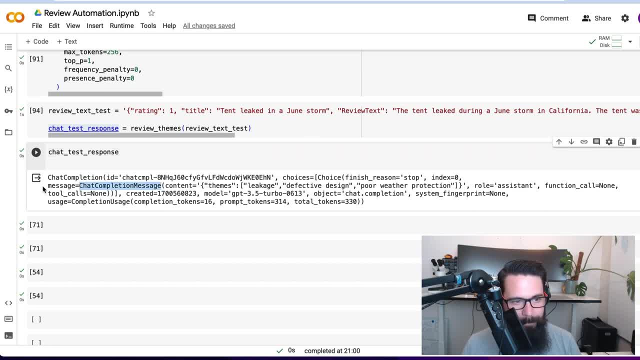 need to say: okay, i, i basically want. where are we? i want the message, the message- i don't think i can get straight to message. we have to go to choices. so why don't we go- and this is pretty cool- dot choices and then from choices i could see that there could be multiple. in our example there's. 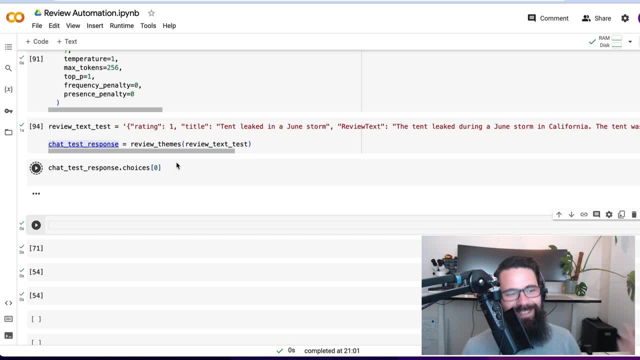 only ever one. so we're going to go open square brackets, zero, uh. and then we've got a choice, and then we've got a message, and then the message has some content. so why don't we see if we can get to? i was gonna put in square brackets, but we'll just 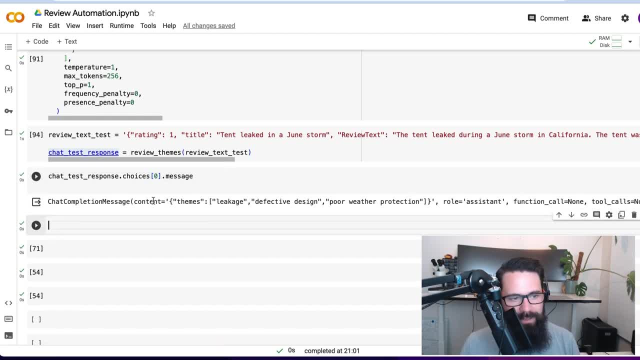 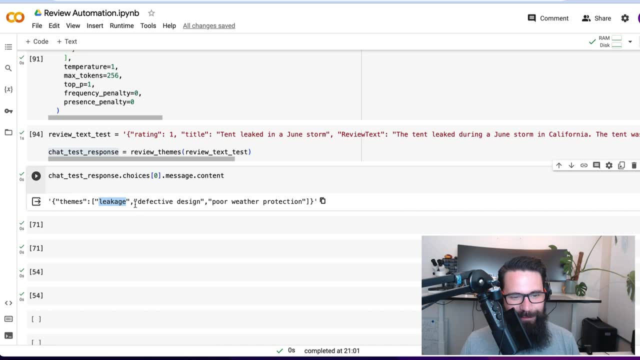 keep with the theme, we'll go: dot message, perfect, and that message has some content. okay, dot content. oh, this is cool. okay, so it's come back with some themes: um leakage, defective design, poor weather protection and the defective desire. like that's just your opinion, man, but you know. 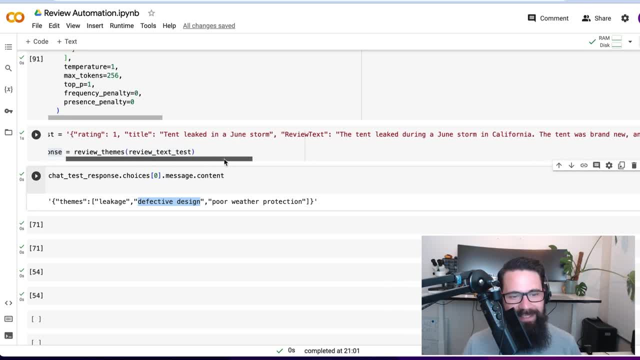 well, let's read the review and understand what's happened here. so tents leaked in the june storm- that was the um the title. the tent, uh, leaked during a june storm in california. the dent was brand new and set up properly by experienced outdoors people, to their credit. let's have a look what's going on here. the leak was in two places, okay, so leakage- perfect- was in two places. and the door zipper. the zippers aren't protected by any kind of waterproofing flap and the rain flyer does not extend to cover the doors. so defective design is probably true and it's. 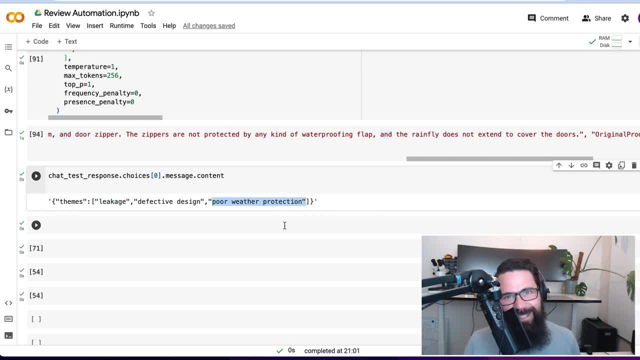 poor weather protection. so it's kind of the things you want a tent to do now. this is awesome. i'm really excited. one kind of bit of cleanup i might do is i might up. i'm actually. i was going to say let's update our function to return this part, but again we're doing it. we're iteration one. 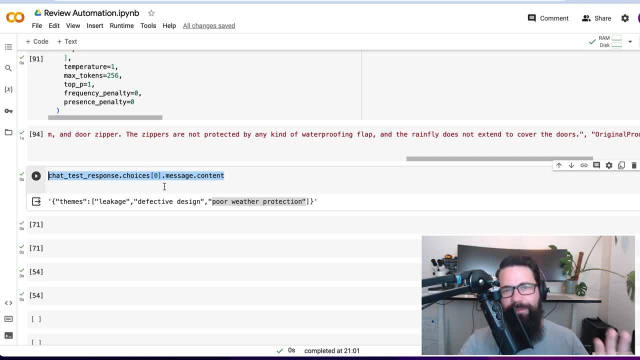 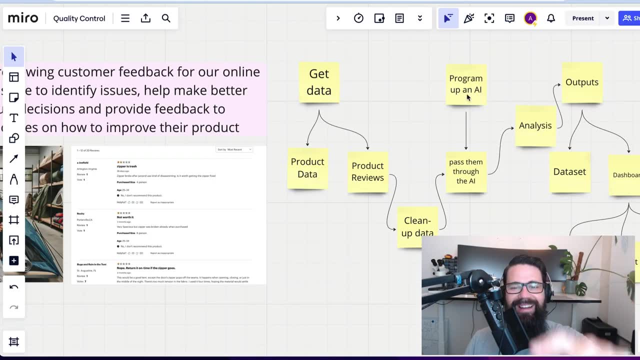 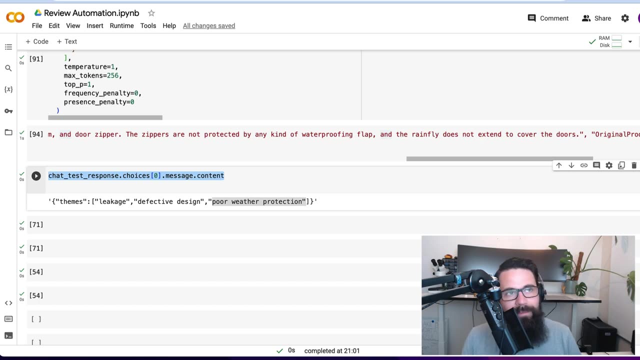 we're doing some real basic discovery. this doesn't have to be perfect. we just need to make sure that every part of our sort of plan- getting the data, product data, review data, cleaning the data and programming the api and passing through to the api- is working and feasible and feasible it. 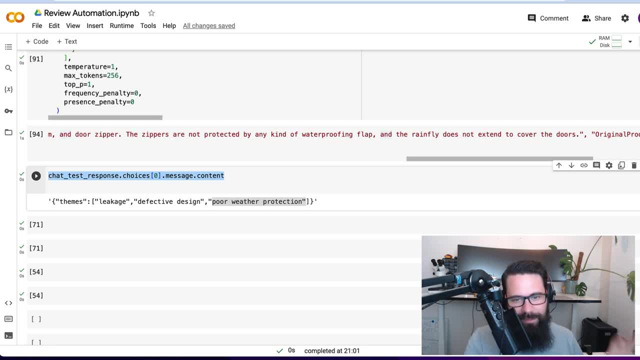 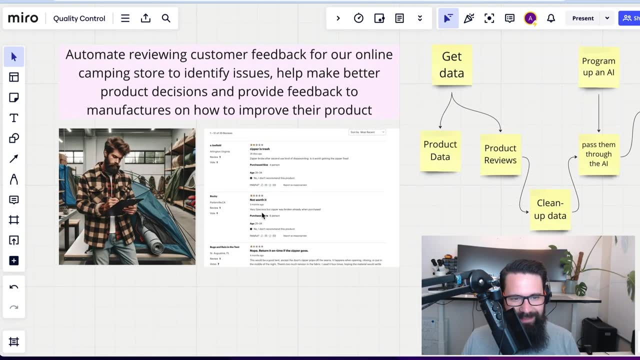 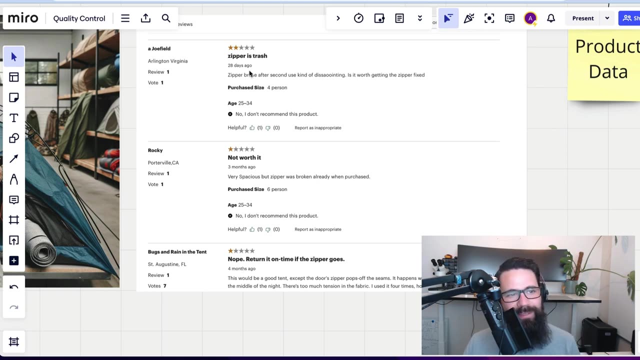 feels like we can sort of get some data out of it and then we'll go back and refactor. so where to from here? now i've got a burning question. if i was to pass in a particular product, this particular product, zipper is trash, not worth it. you know, these type of reviews will i get back? 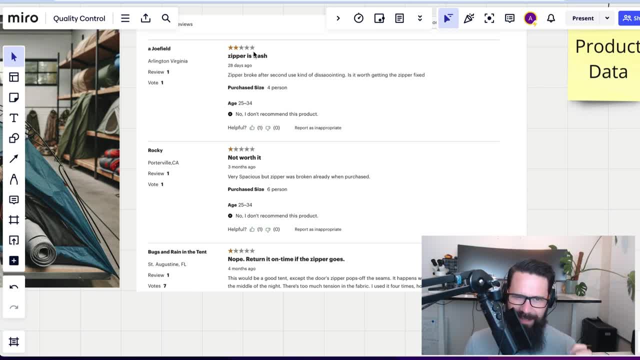 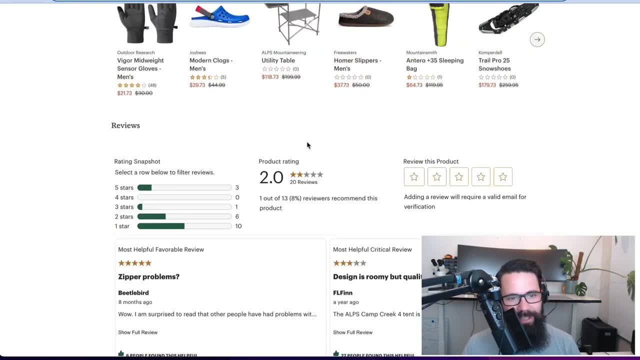 the zipper comment, or do i need to tweak my system message? do you really get that level of detail? so how do we do that? so let's go back to the actual website, and this is the listing that has all the really uh poor zipper reviews. so why don't i go ahead and take from the url the product id and 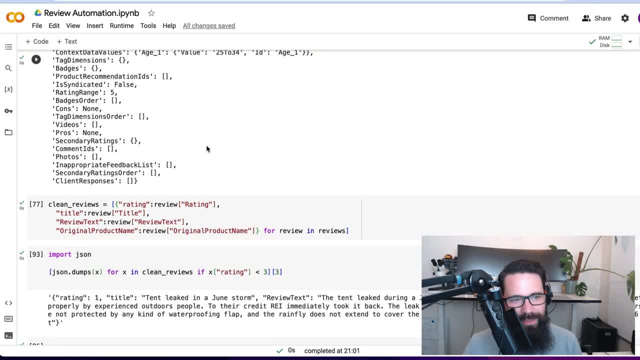 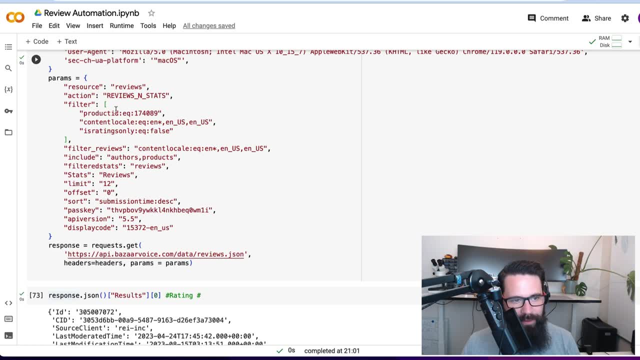 you can tell i'm getting a bit excited about this and what i'm going to do is i'm actually going to go ahead and update my system. so i'm going to go ahead and update my system. so i'm going to go ahead and update our reviews api call, which is this one here where it says product id is equal to. i'm going 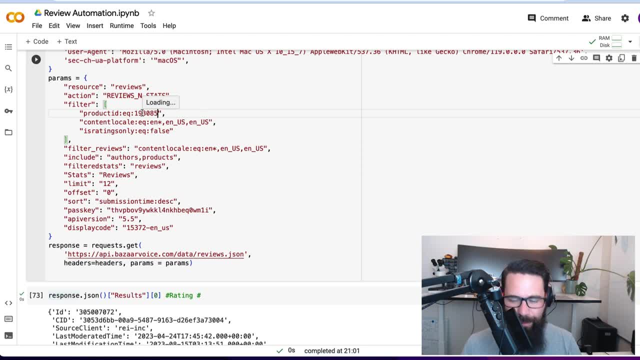 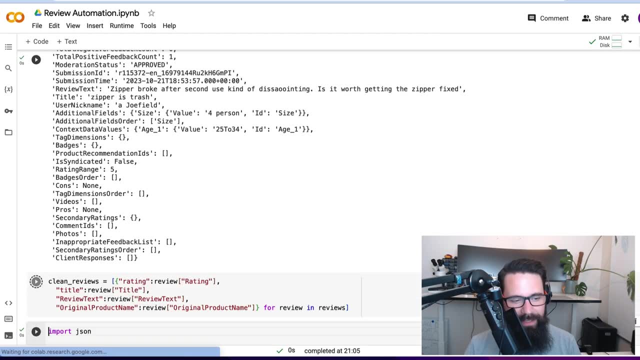 to paste in our product with the known issue, the zipper issue. okay, so we've got our product id in there. okay, we're going to run this, perfect, and we're going to run this and we're going to run this and we're going to run this and we're going to run all these, and then now we've got is we've. 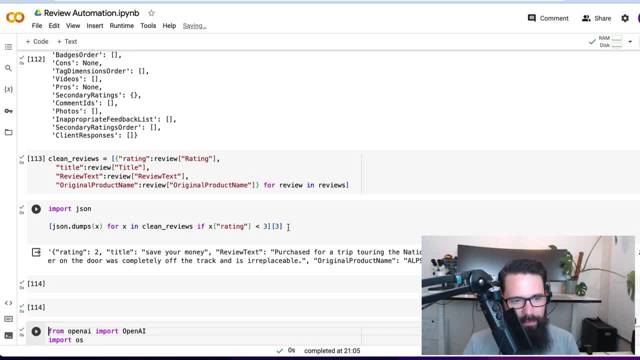 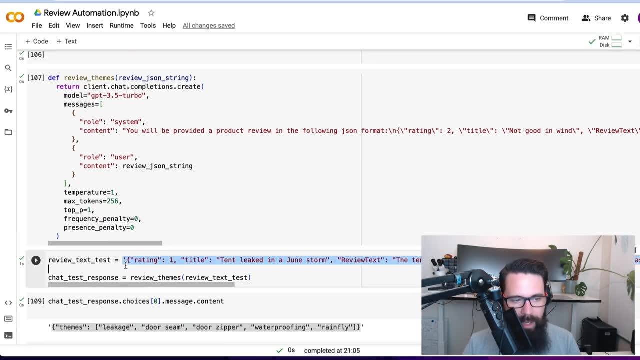 got this particular one here. so what i might do is i might copy this out and if i scroll down, if you're going to copy this out and if i scroll down, if you're going to copy this out and if i scroll down, i had just static text in our review text test. i'm going to paste this in here because this: 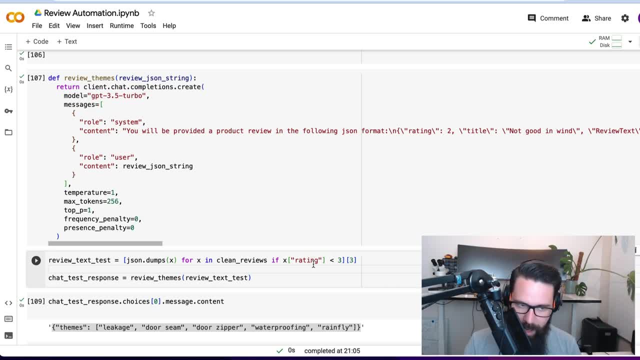 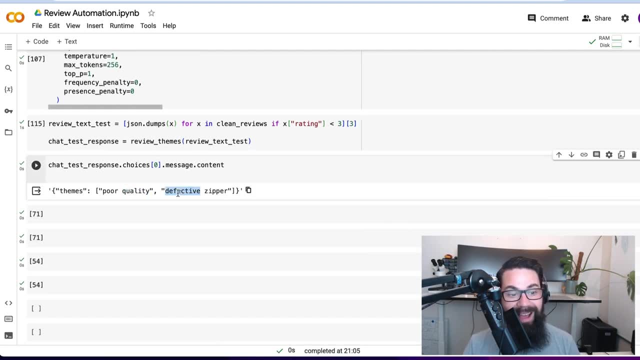 is from above, where we know it's about the zipper, and i'm going to shift enter and shift enter on that scroll down and what i'm hoping- ah, perfect, defective zipper. that's all i wanted to see. but how well is it? so we know a lot of these reviews are about the defective zipper, so why? 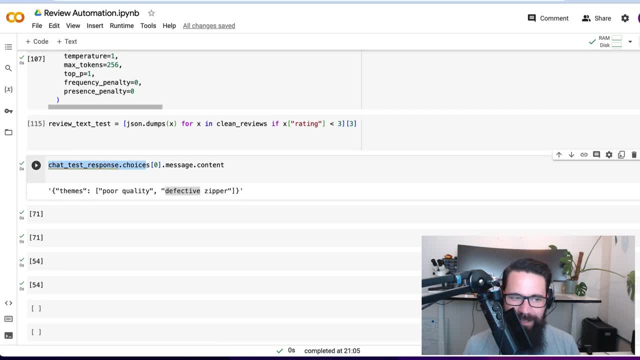 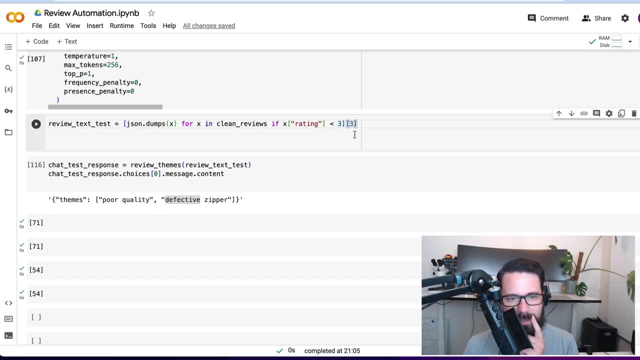 don't we do some tests on that? let's test a little bit more, just to make sure i'm not getting carried away and too excited for something that isn't true. so what i might do is to really test this is i might loop through the first three. no, actually take it. i'm getting carried away, we're. 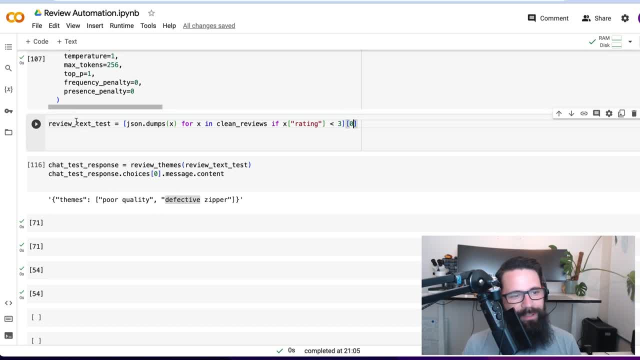 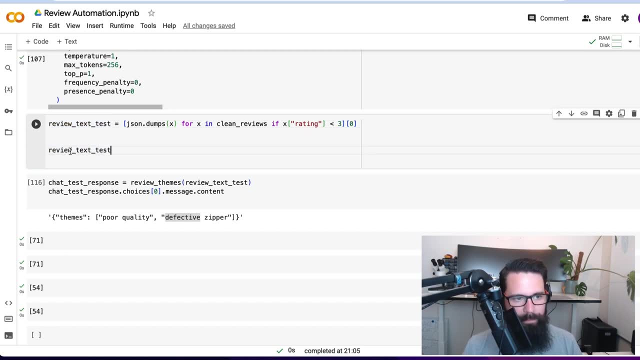 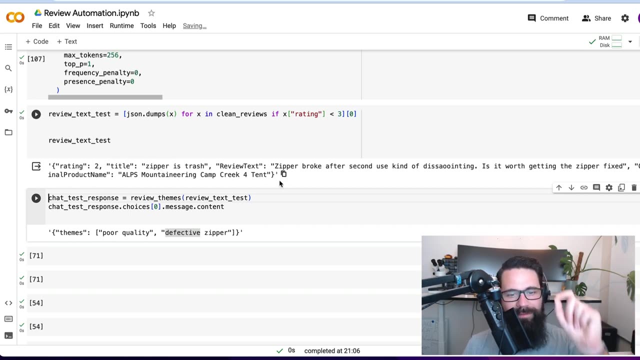 not automating the whole process, we're just testing. so let's have a look at the first piece of text. okay, let's have a look at that. so copy that paste. where are we paste that shift enter. now what do we got? so we've got a rating. two: zipper is trash. zipper broke off after second use. 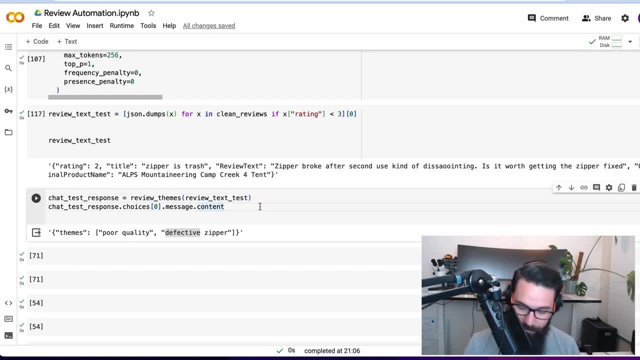 kind of disappointing. yeah, i'd be disappointed too. so if i run that piece of text through chatgpt, do we get? oh, zipper quality? yes, yes, that's the first one. perfect, okay, let's keep going. should enter on that. uh, not worth it. uh, very spacious, but zipper was broken. let's run it through. 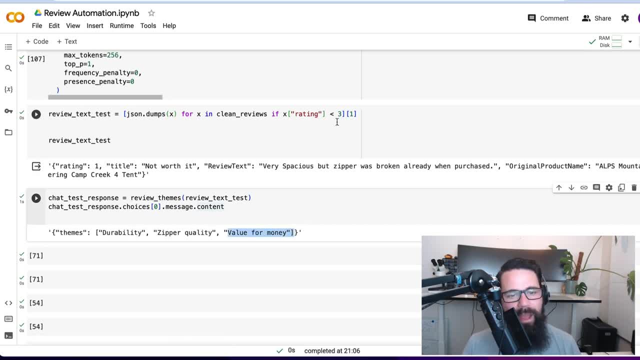 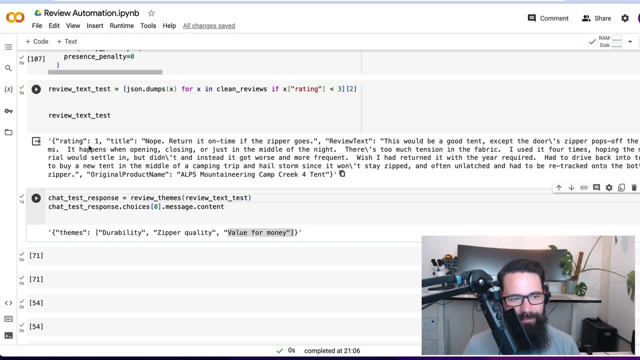 durability, zipper quality and value for money. uh, and we did, we're done through. or let's go two? okay, We've done three. Oh, let's go two. Okay, perfect, Let's go one more. If we get zipper on this one, then I'm going to be happy. 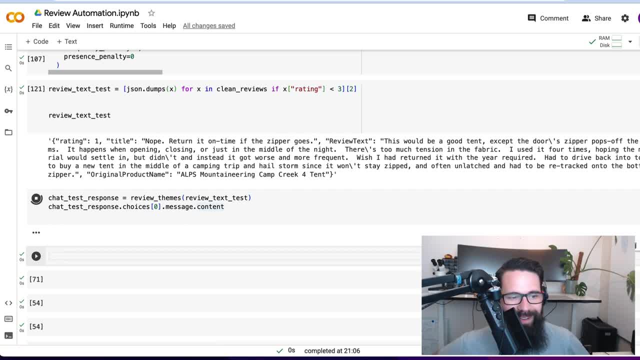 Well, yeah, zipper is gone, Okay, perfect, So let's run it. What do we get back? Zipper, quality, door functionality, fabric tension, return policy, durability, Perfect, Amazing, Okay, great. Where are we at? 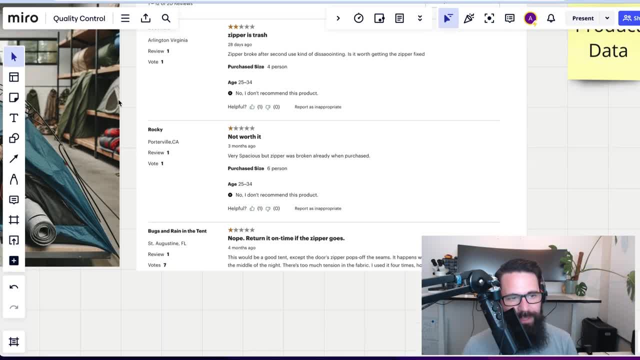 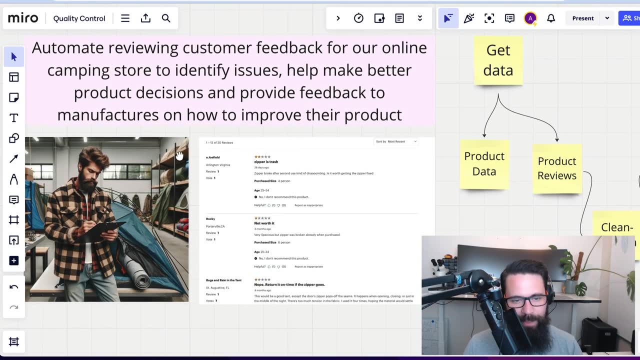 So, end-to-end data analysis, Are we ticking the boxes? Are we doing everything we are setting out to do? So, going back to the beginning, what we're trying to do is help automate this guy with the good hair from the AI image generator: the ability to review thousands of product. 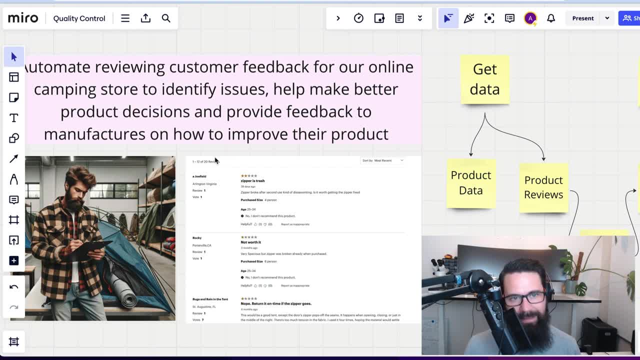 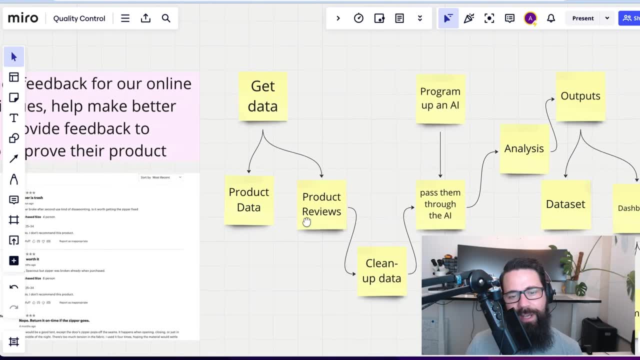 reviews and extract key themes that are causing customer pain. Can we do that? So let's check all the boxes. Can we get the data? So far, it looks like we can. We've got some data, got some product data, got some review data. 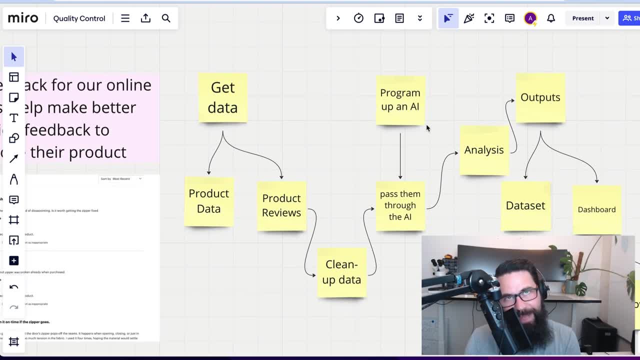 We'll clean that up. We have programmed up our API- AI API- through the system messages and through Python, and we've actually tested passing through a number of those. We've also tested passing through a number of those through to AI, which is awesome. 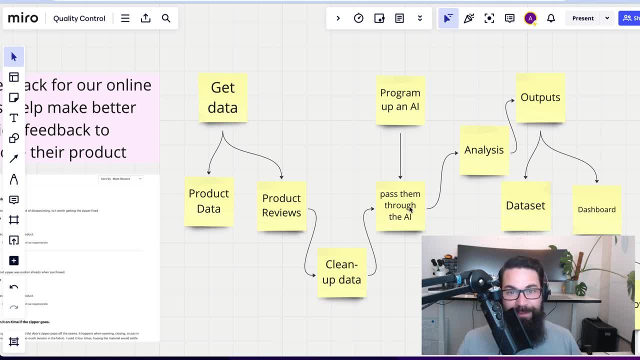 We are. we're in a really good place. So from here, well, first of all, make sure you subscribe, because I'm on a bit of a roll with these videos. I want to take you through that full end-to-end sort of analysis and make sure, yeah, you're. 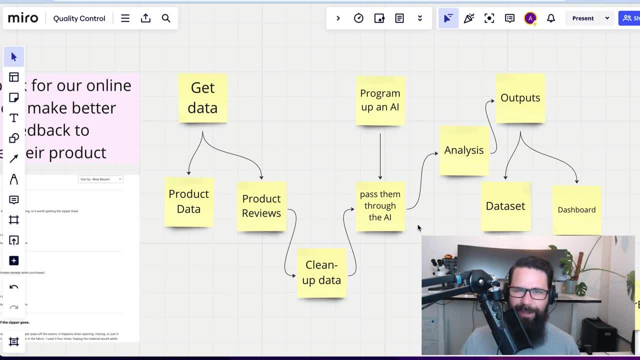 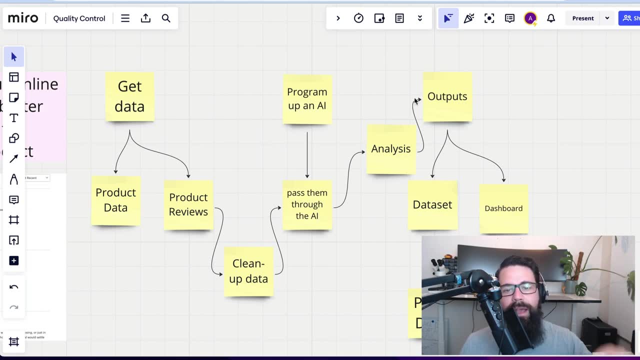 subscribed, got all your notifications. whatever else you need to do is turned on. If this is useful, drop a comment. If it's not, also drop a comment. I love to hear from people who have feedback. After this, we are going to the next video. 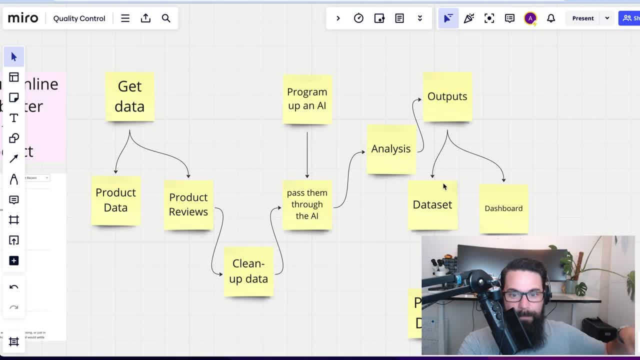 We are going to go through our analysis. We're going to look at some of the main outputs. One's going to be pretty plain text output, some data sets. The other is going to be some dashboards. but there is one step I want to add it.